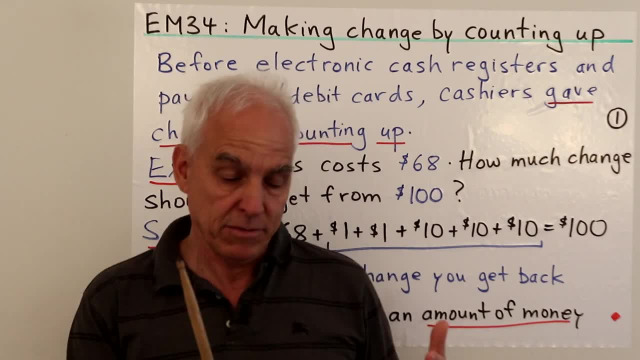 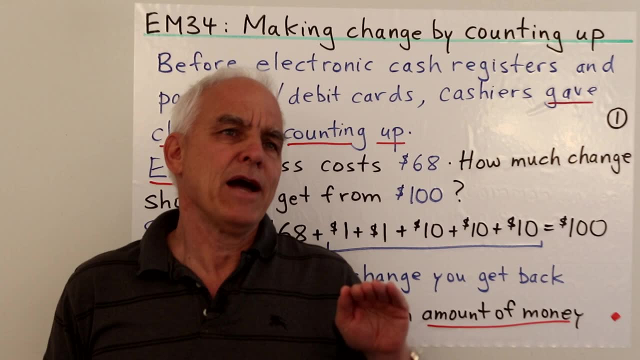 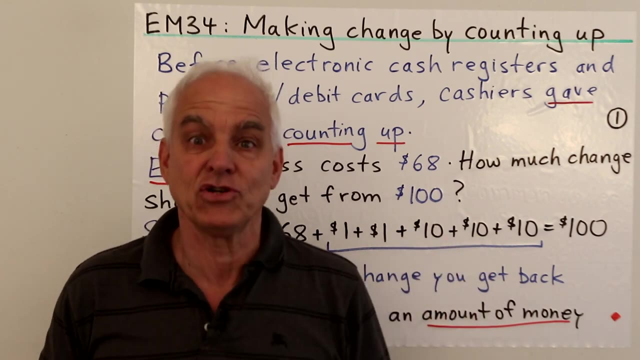 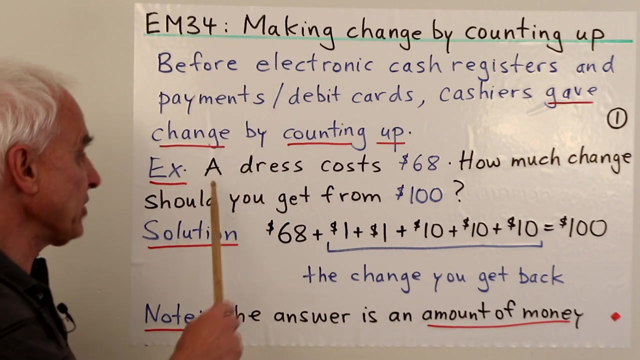 technique to teach young people, strengthen their arithmetic And also connect with money. And we'll see that there's a side benefit that we are touching base with the decimal aspect of dollars and cents, which is a great introduction to decimal numbers, kind of a first steps in that direction. So, for example, suppose that you go into a store. 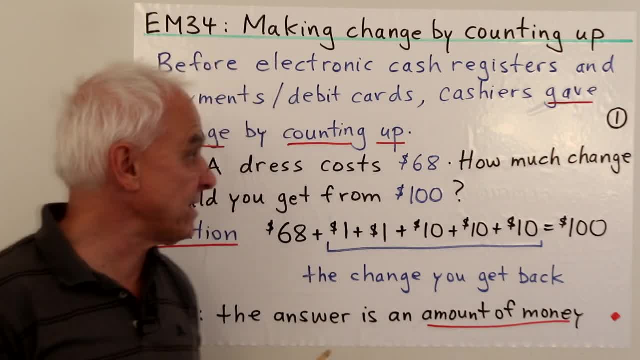 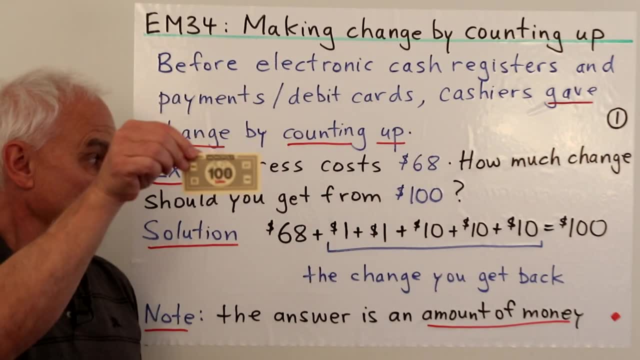 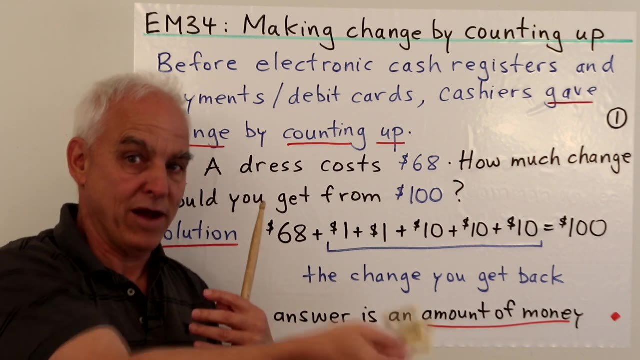 there's a dress. you're going to buy this dress. It costs $68. And you're going to pay with a $100 bill. So there's $100.. You give the $100 and you're going to get the dress, but you want. 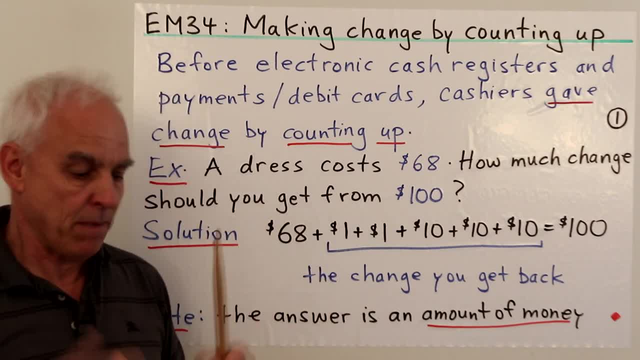 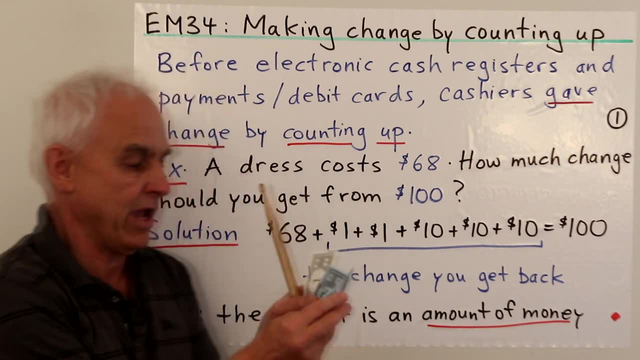 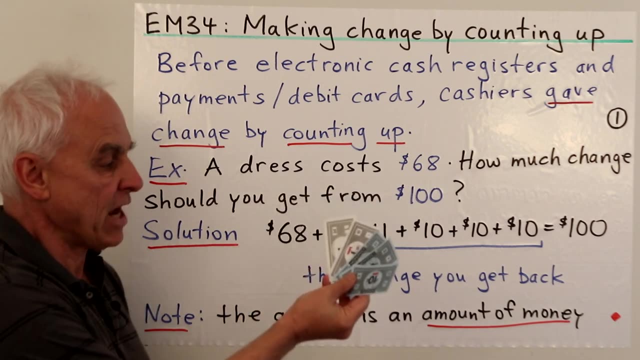 some change from your $100.. So what's the shopkeeper going to do? Well, what they're going to do is they're going to prepare some change. This is actually the amount of change that they're going to give you. So they figure out what this is one way or the other, and here's how they give. 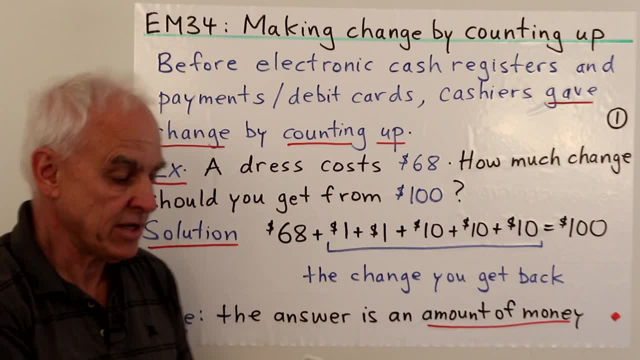 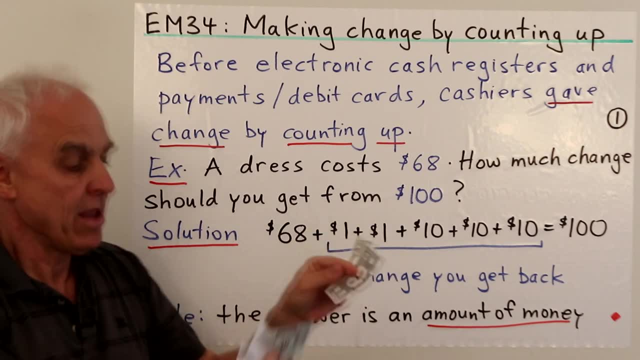 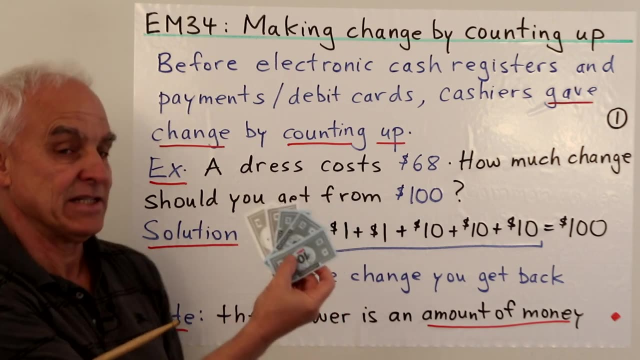 it back to you, They might say: okay, the dress is $68.. Plus one is $69. Plus another one is $70. Plus 10 is $80.. Plus another 10 is $90. Plus 10 is $100. So we've started with the cost of the item and then we've added. 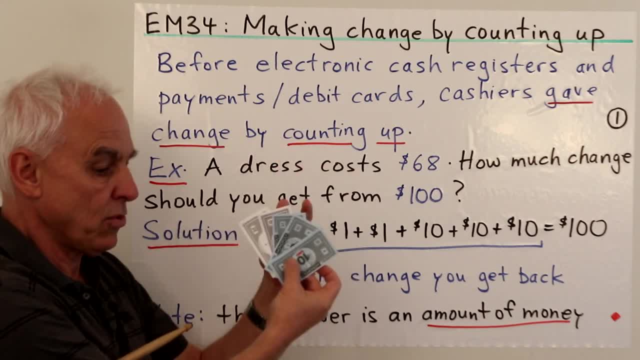 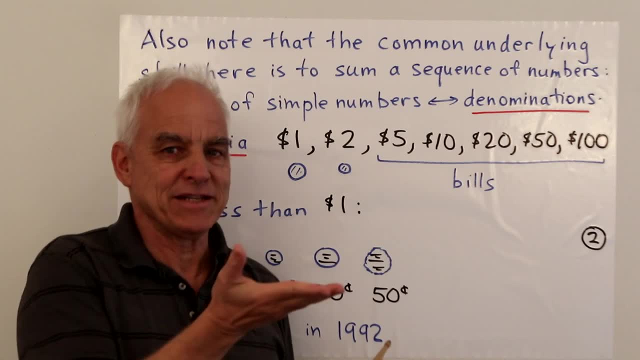 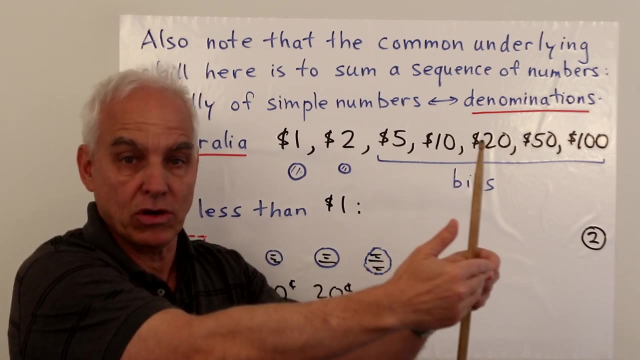 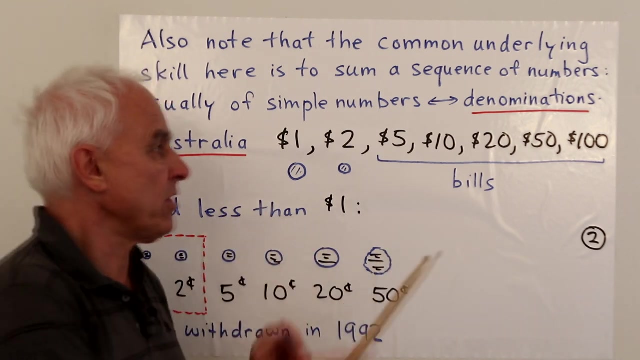 the various monies to get the total of the $100 that you paid. So the underlying skill here is still the fundamental one of being able to add a sequence of numbers and keep a running total of the amount. Usually the numbers that we're adding are simple numbers and associated with denominations of actual money, that is. 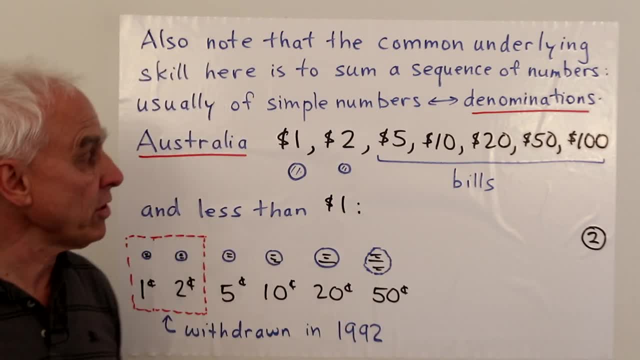 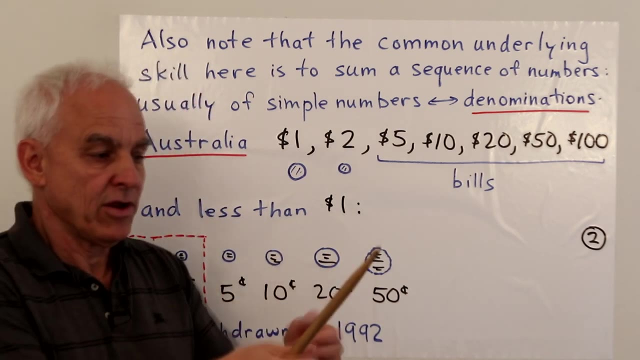 involved. So in Australia the currency in terms of dollars is in terms of some bills and coins. We have a $1 coin, a $2 coin, And then bills of $5,, $10,, $20,, $50, and $100.. So, in actual practice, returning change would 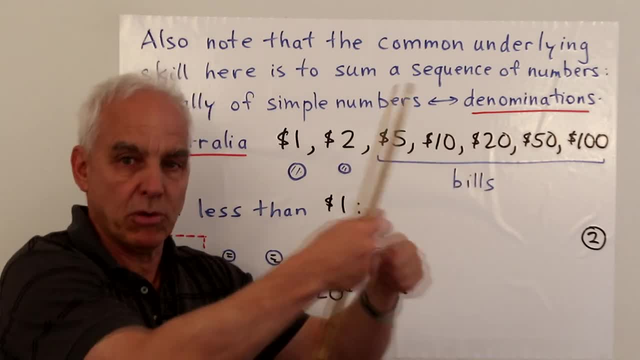 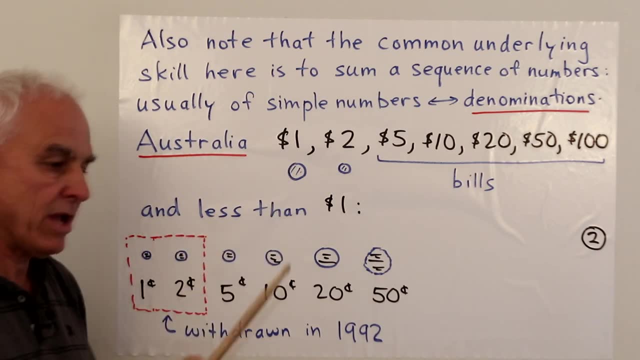 typically involve these kinds of numbers. These are the numbers that would be typically added up. Of course, there's also the smaller numbers, So less than $1,. we have smaller coins. We have- well, we used to have- $0.01 and $0.02 coins, but these are no longer in circulation. They. 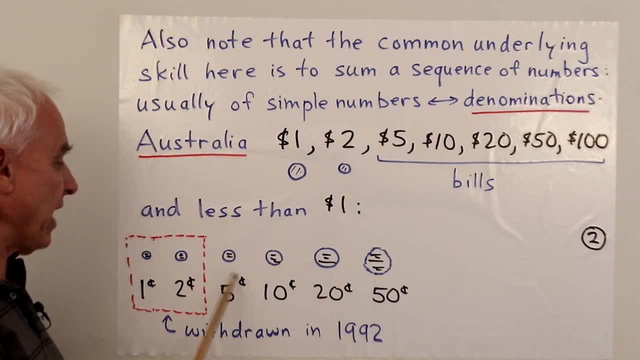 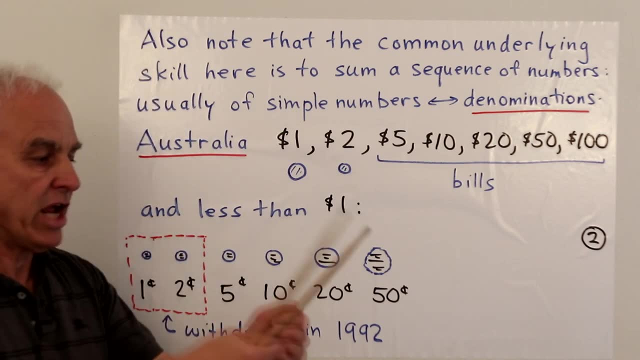 have been withdrawn. So the smallest actual coin that you typically find is a $0.05 piece. There's also a $0.10 piece, a $0.20 piece and a $0.50 piece, So making change typically involves a combination of coins and also of bills. 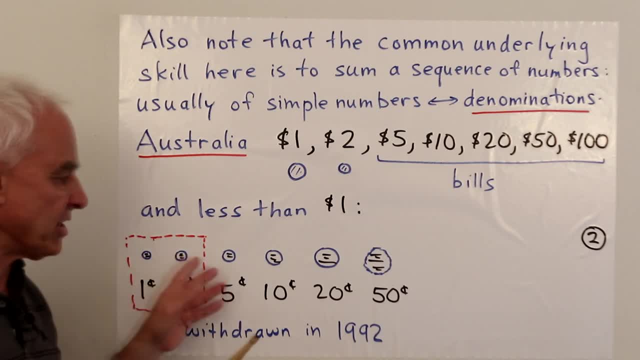 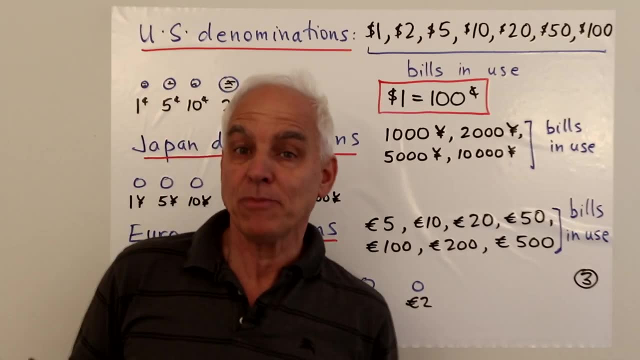 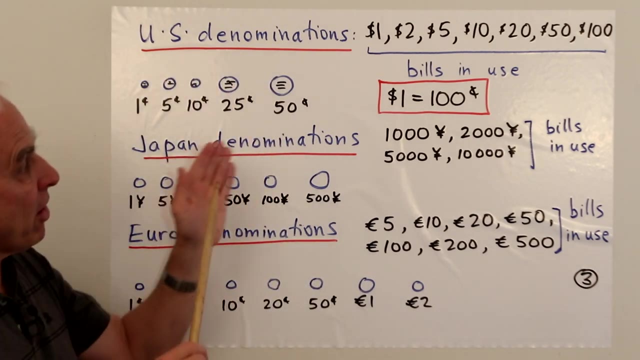 So this counting up process actually does incorporate both of these cents and dollar amounts. This is also a good time to remind ourselves about different currency systems around the world. This is also a good time to remind ourselves about different currency systems around the world. So in the United States, here are the kinds of monies that are typically in use. Here are the best. cut work at the moment. So the bills in the United States are $1,, $2,, $5,, $10,, $20,, $50 and $100.. There are actually also some bigger bills. there's a $500 bill which is no longer used in ordinary. 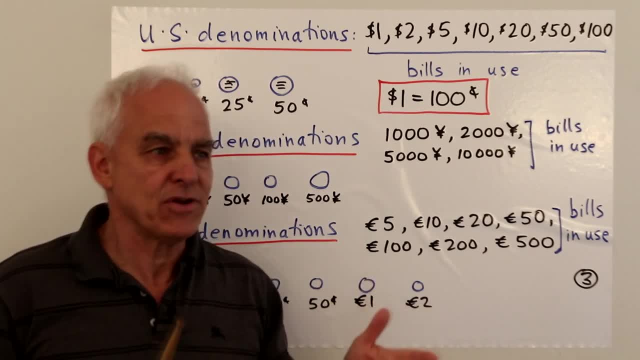 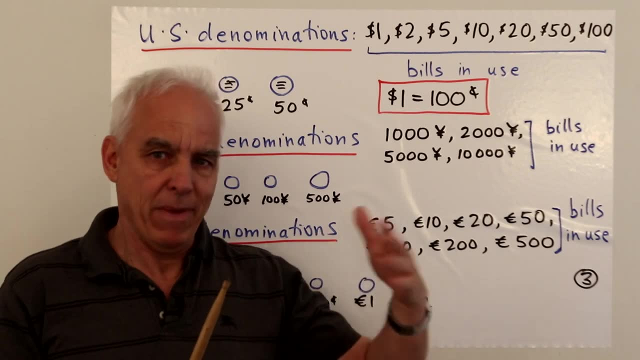 circulation, but there's also actually officially also some. some larger bills, probably going up to maybe a hundred thousand dollars, May be used in bo totals of 100 with this hit money. does it favor? the maybe are more the domain of banks, so banks can use these bills. they're actually a legal tender. 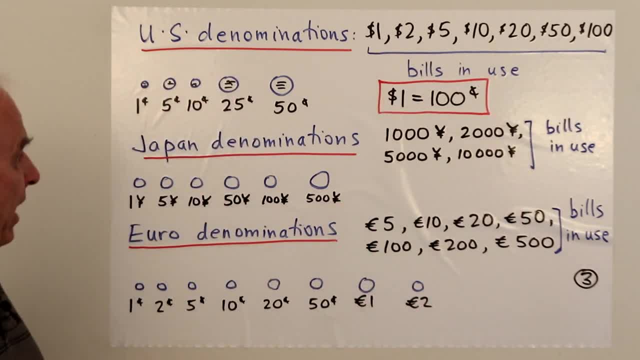 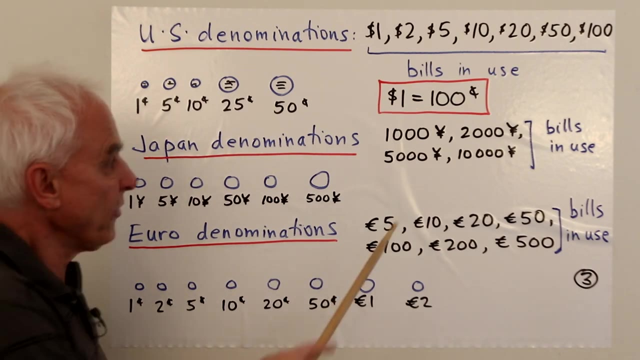 but in ordinary usage up to a hundred dollars is the max. and then the coins: there's a one cent coin, five cent coin, ten cent coin or a dime 25 cent coin or a quarter. in japan, where we have yen, the bills are 1 000 yen, 2 000 yen, 5 000 yen and 10 000 yen. and the coins are 1 yen, 5 yen, 10 yen, 50 yen, 100 yen and 500 yen. so very roughly, 100 yen is somewhat comparable to a dollar in the eurozone. the bills are 5 euros, 10 euros, 20 euro, 50 euro. 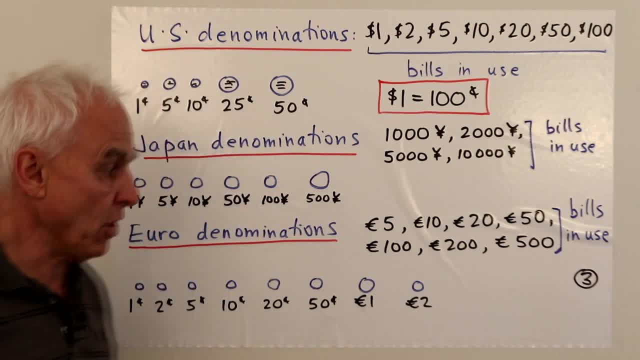 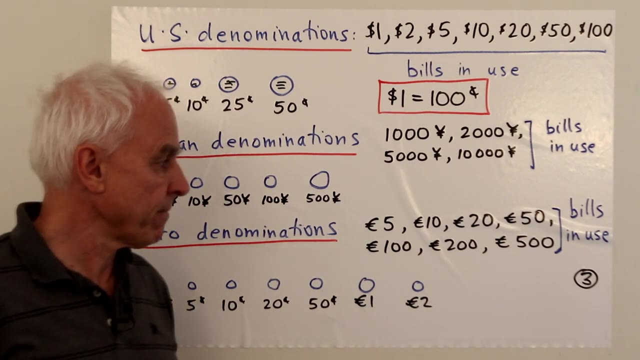 100 euro, 200 euro- and this is a 500 euro note- and the coins are one cent, two cents, five cents, 10 cents, 20 cents, 50 cents and one euro, which is like 100 cents, and there's also a two euro coin. so giving change in these various different places would look different, because you're actually using 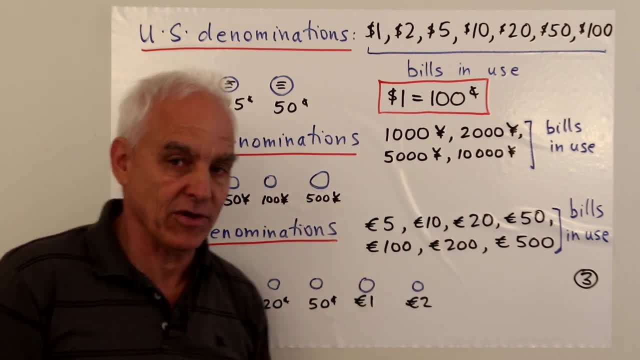 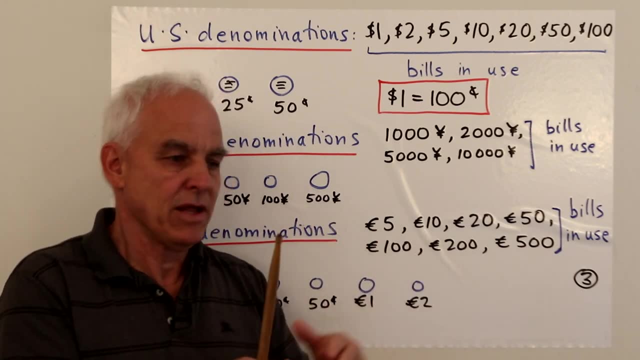 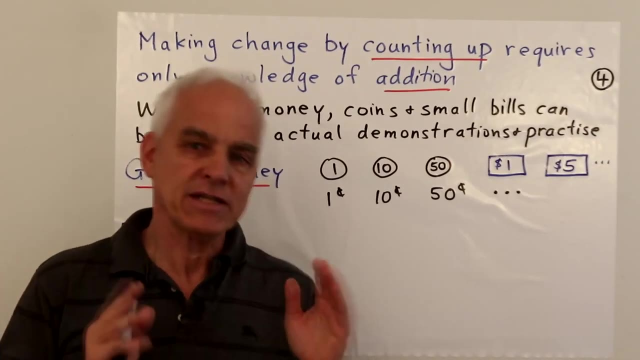 the various currencies and, of course, in other countries. there's a wide range of things, but we're going to kind of focus on the dollar situation. typically, then, which consists of 100 cents, makes a dollar. so, as i've said before, this technique of counting up requires mostly just 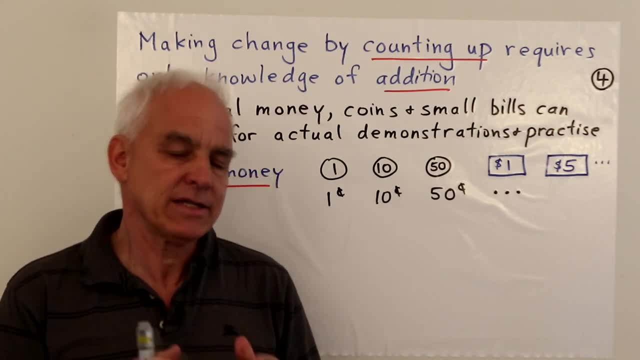 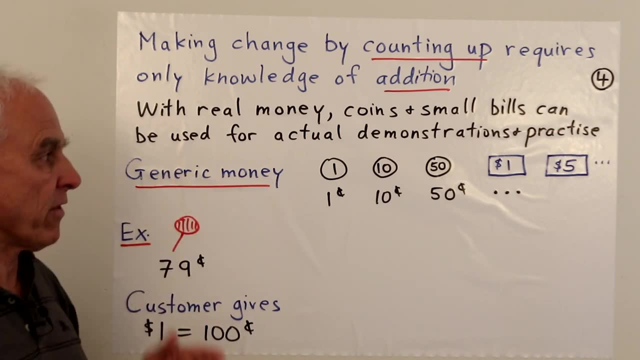 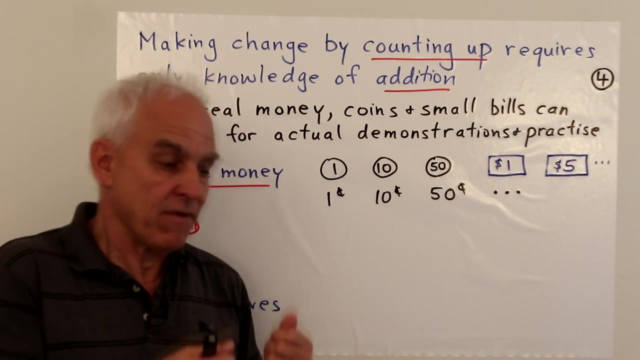 addition- actually subtraction isn't really explicitly involved. okay, so, with real money, coins and small bills can be used for actual demonstration. so if you actually have a classroom with some children or you're teaching your children at home, it's fun to use actual money. but of course you can also use monopolies. 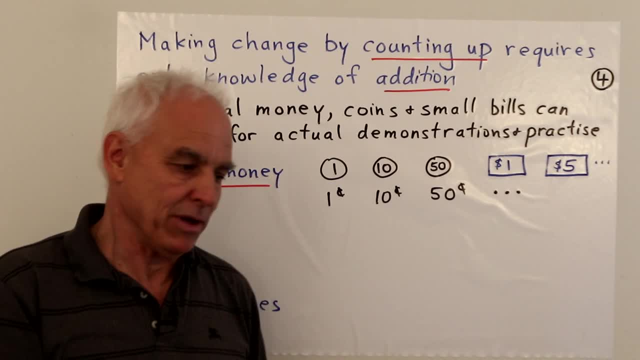 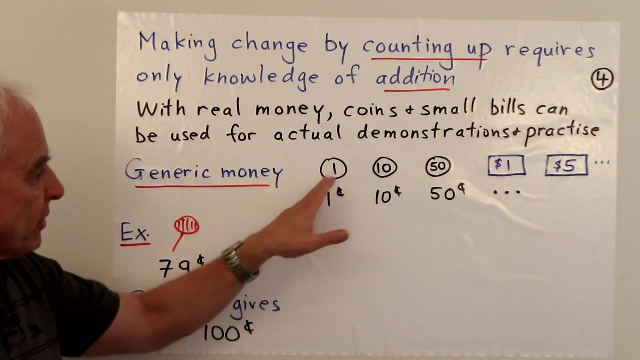 money. so if you're talking about dollars, it's probably practically better to have monopoly money, but with coins you can use just coins around, okay. so it's actually good to do this physically and directly. so, to illustrate things, we're going to sort of use some generic money. 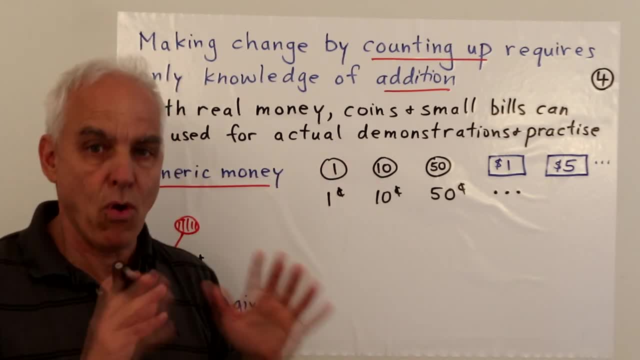 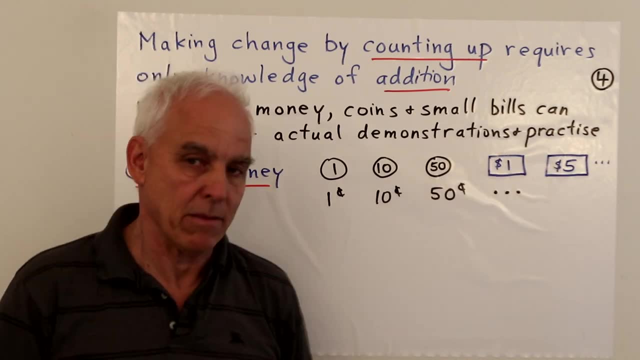 so whenever i make a little circle with a number in it, that refers to coins, with the idea that these are cents, and whenever i make a little rectangle like this, we're talking about bills, typically dollars. okay, so let's illustrate it with a simple example. here is a. 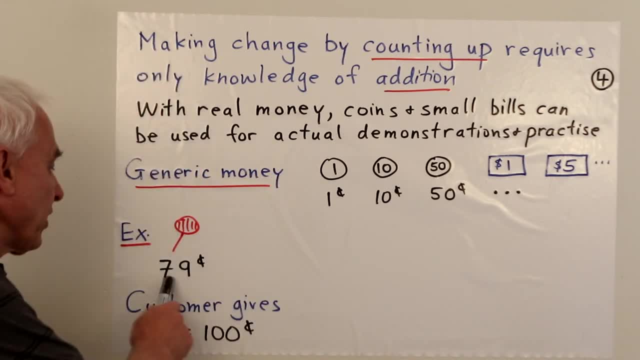 piece of candy and a child goes into a store. the candy is worth 79 cents, let's say, and the child maybe gives the store owner a dollar which is 100 cents. okay, so what should the child get back from their dollar if the candy costs 79 cents? well, the store owner gives them back one cent, okay. 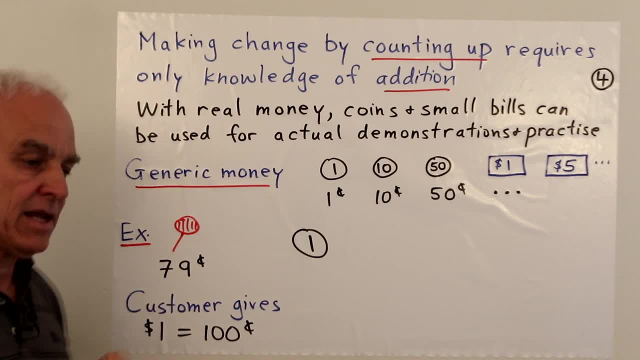 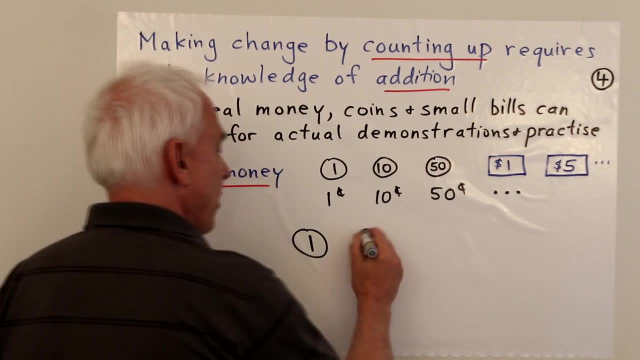 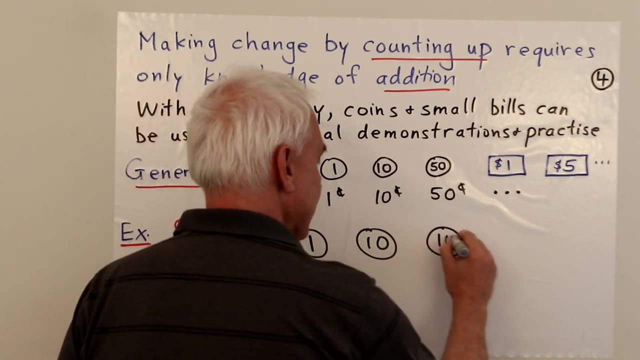 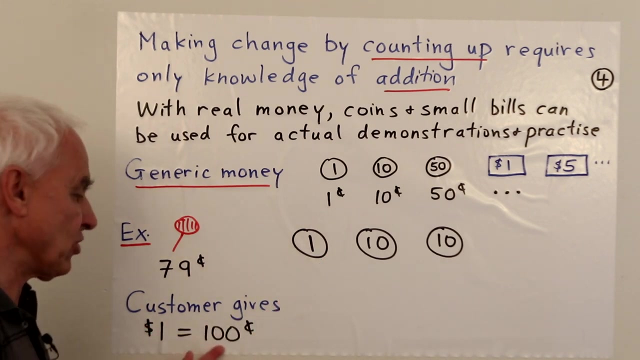 so one cent, together with the candy is then a total of 80.. so 79 plus 1 is 80. and then another 10 makes 90 and another 10 makes a hundred. so now the total amount given back is equal to the total amount received. so the process is finished and this is the amount of. 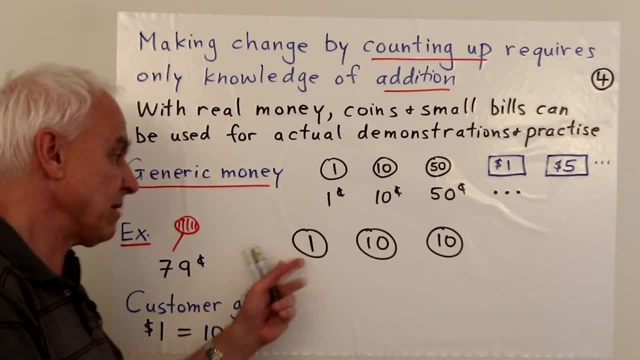 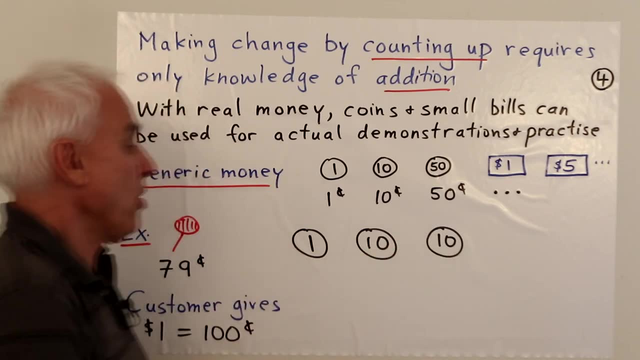 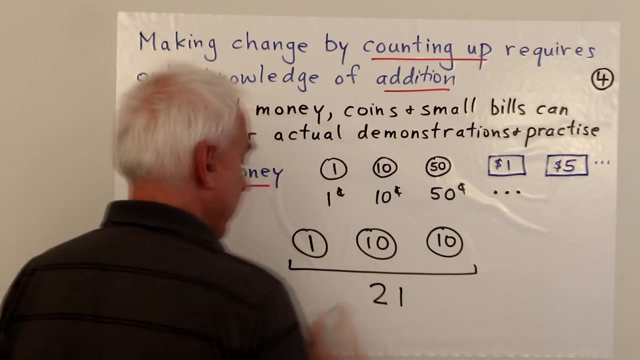 change that the child should receive one cent piece, a 10 cent piece and another 10 cent piece. of course, the child can then say: okay, well, the total here, the total is 1 plus 10 plus 10, which is 21.. and this then represents the equation, that's 79 cents plus 21 cents equals 100. 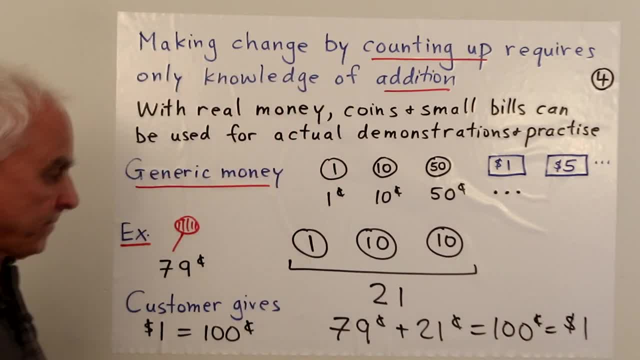 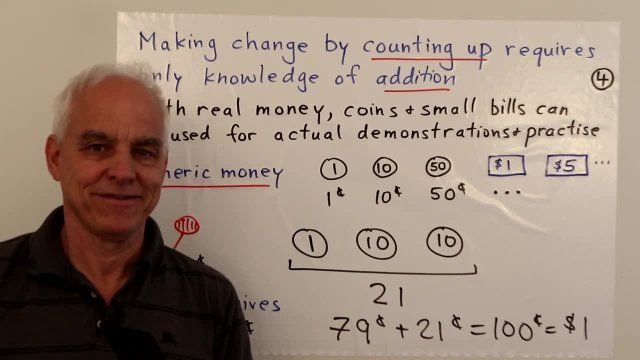 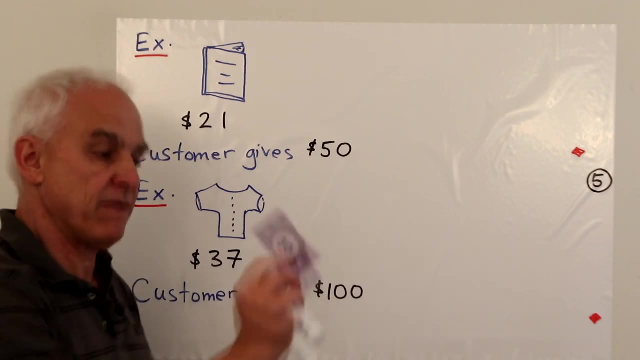 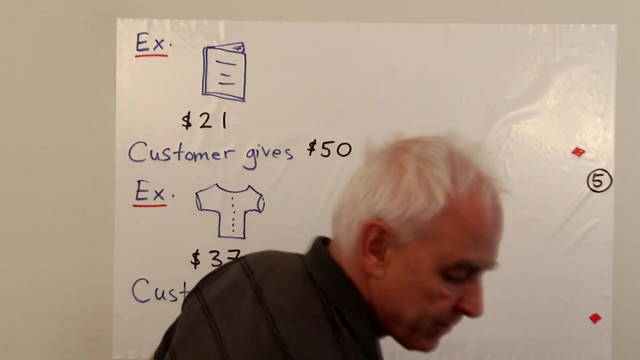 which is the one dollar that was given. so this is the underlying balance that's represented by this transaction. all right, so with our next example, suppose that a book costs 21 and it's paid for with a 50 note. okay, so what should the customer get back? well, we start with 21. 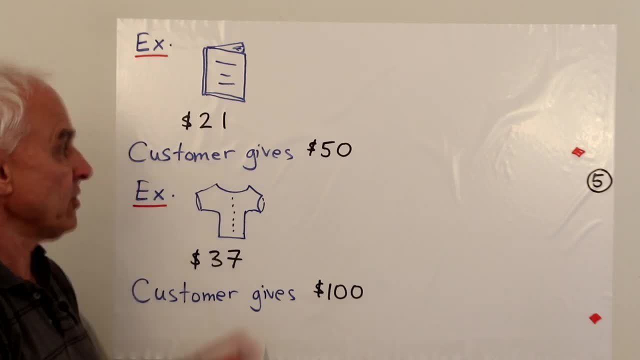 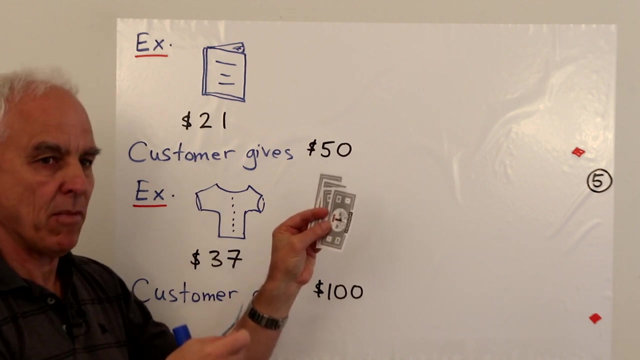 and then we have to count up 250.. so 21 plus 1 is 22, plus 1 is 23, plus 1 is 24, plus 1 is 25.. so we kind of pause there. we've reached a multiple of five, and now we can shift from ones to a bigger unit, namely fives. so we have 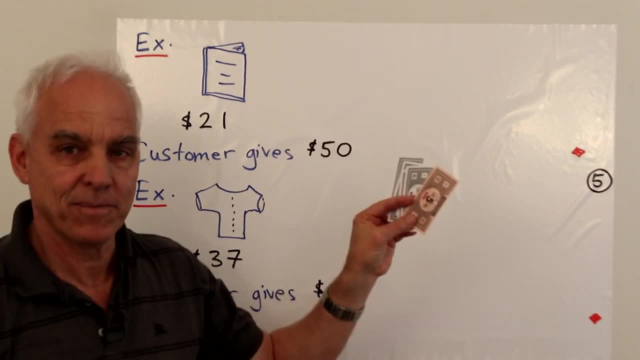 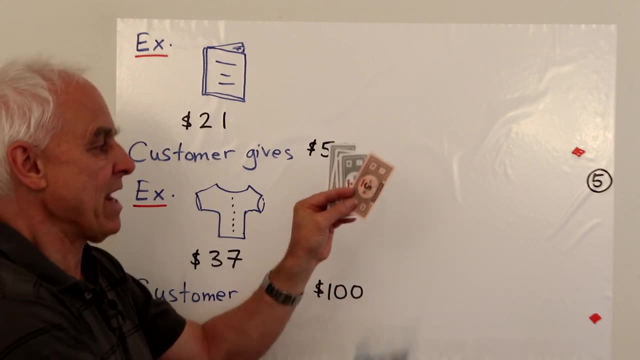 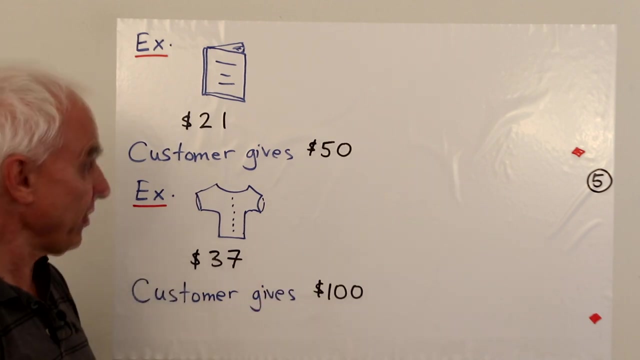 25 all together. now we add 5, that makes 30. now we're at a bigger multiple. we can now add some 10s because we're heading towards 50. we have 30 now. add 10 is 40. add another 10 is 50.. all right, so all together. what's happened is that. 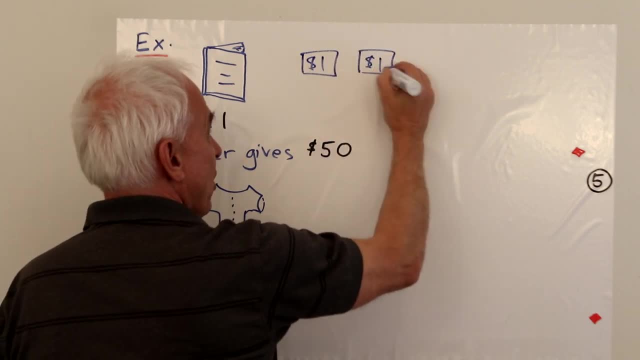 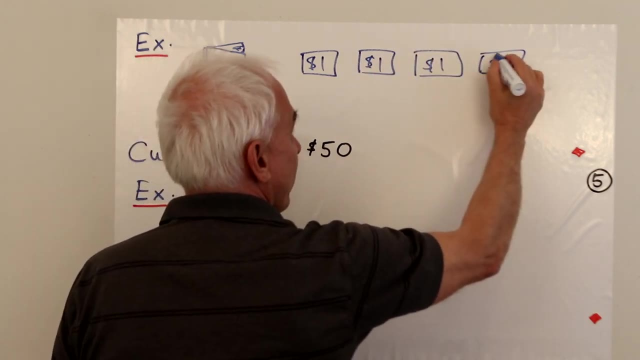 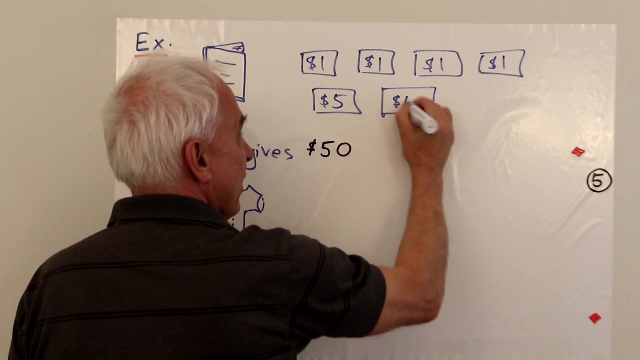 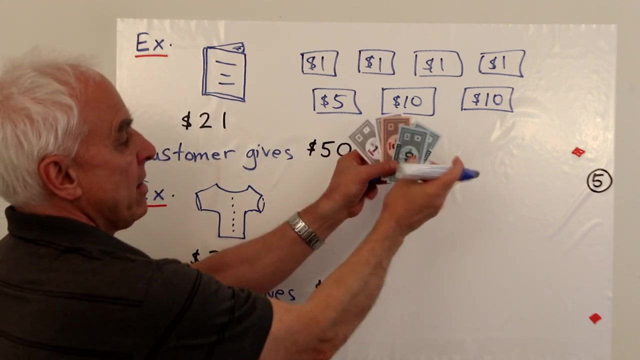 we've gotten back a dollar and another dollar. 21 plus 1 is 22 plus 1 is 23 plus 1 is 24 plus 1 is 25 plus 5 is 30 plus 10 is 40 plus 10 is 50.. that's the total amount of money that's received in change. we've counted up from 21 to 50.. 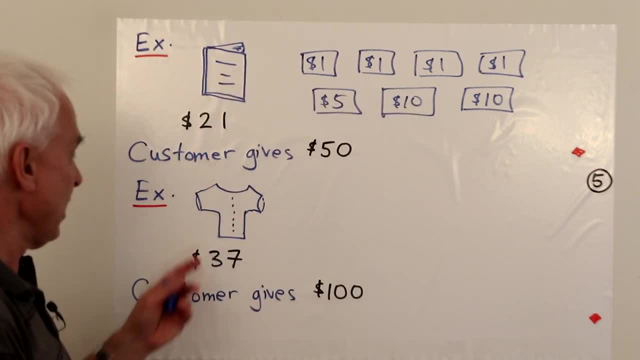 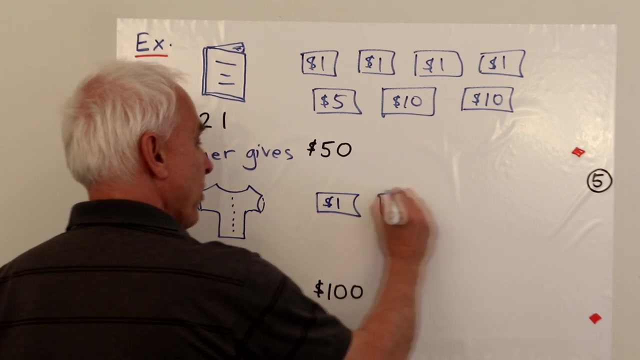 as another example, i'll do it without physical money. suppose that a shirt costs 37 and you're paying with 100. so we have to count up from 37 to 100.. so 37 plus 1 is 38, plus 1 is 30.. 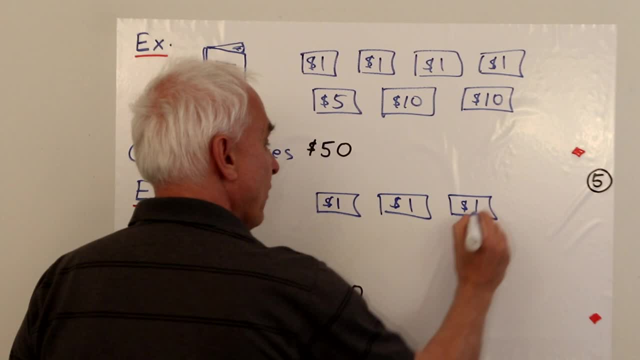 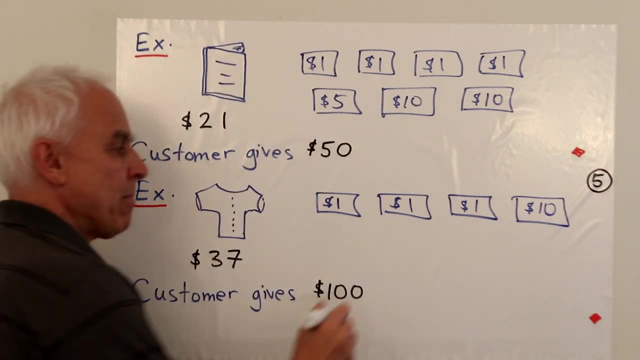 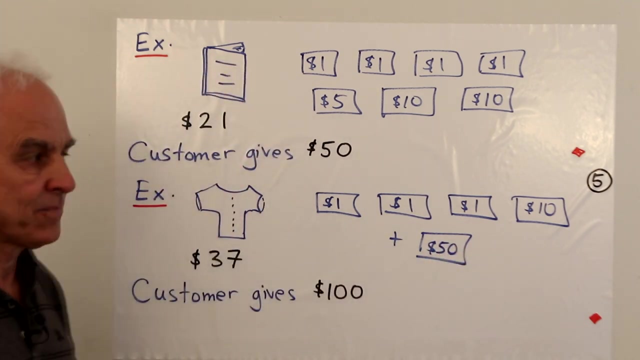 plus 10 is 39 plus 1 is 40 plus 10 is 50 plus 50 is 100, and so out of a basket of three one dollar bills, 1 10 dollar bill, 150 dollars bill is added to the thirty-seven dollars to get a hundred dollars. 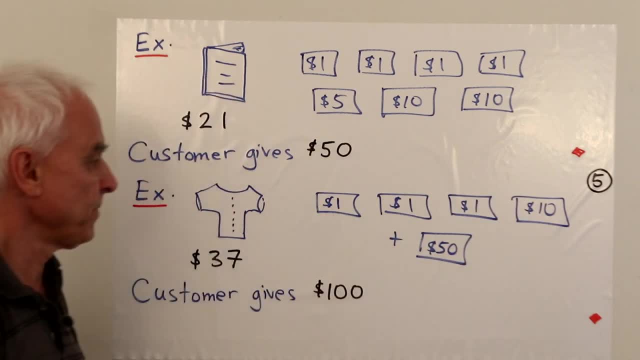 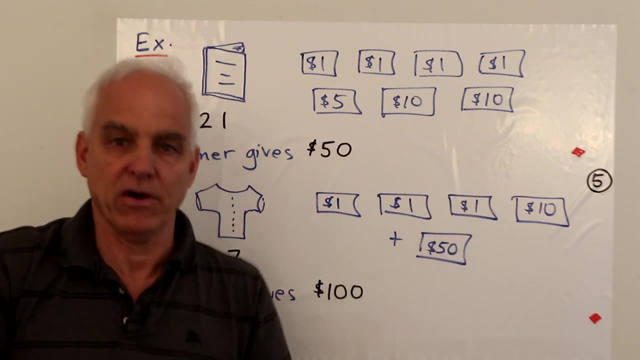 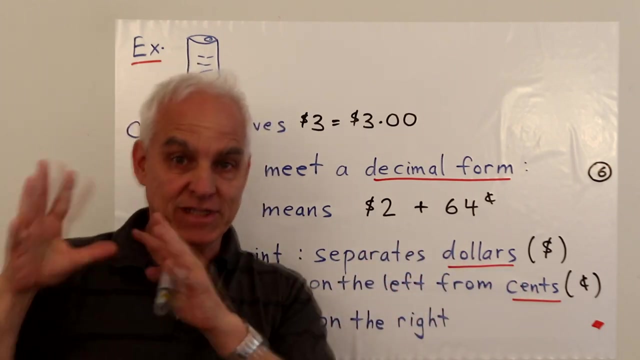 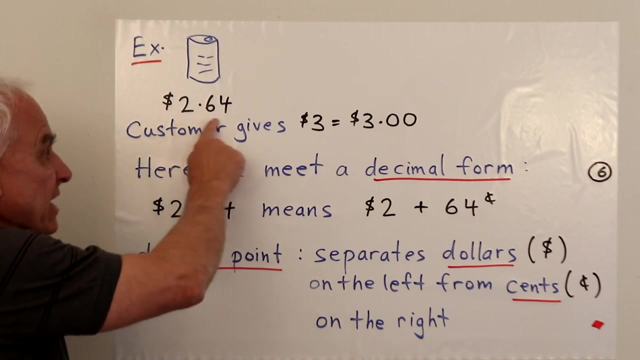 1 amount of change received. we've counted up from 37 to 100 using the, the bills that are available to us in our local system. now, in this example, we are moving into new territory because we're going to mix the cents with the dollars and mathematically that means introducing this kind of decimal. 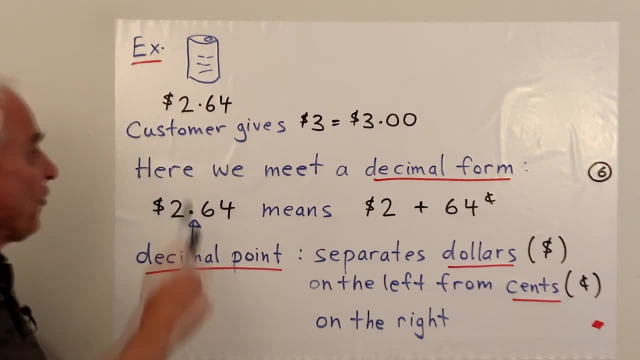 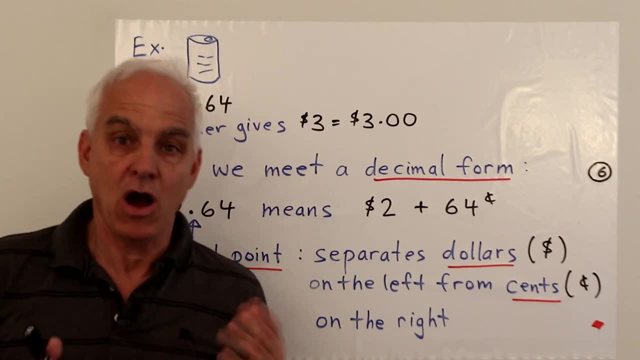 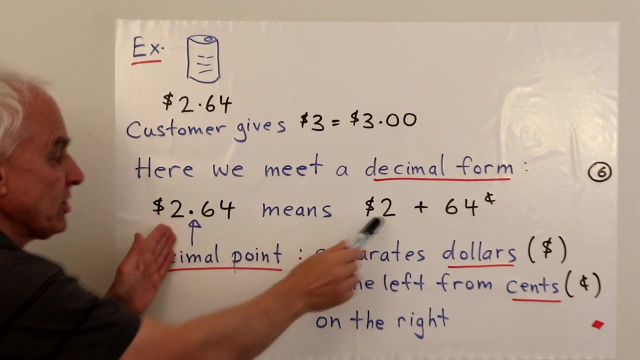 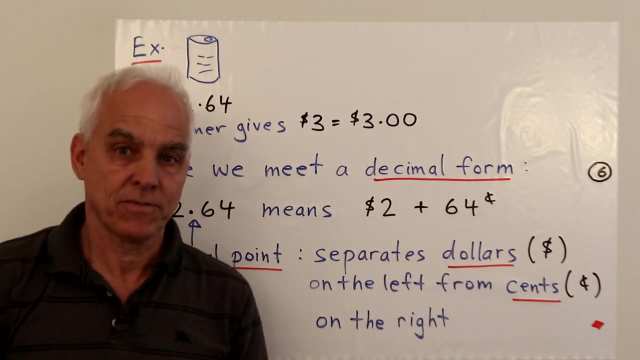 representation of a money amount. so this is 2.64. that's how much this can of drink costs. okay, so the point there, that's the decimal point that separates the two dollars on the left hand side and the 64 cents on the right hand side. this is a very important kind of mathematics. 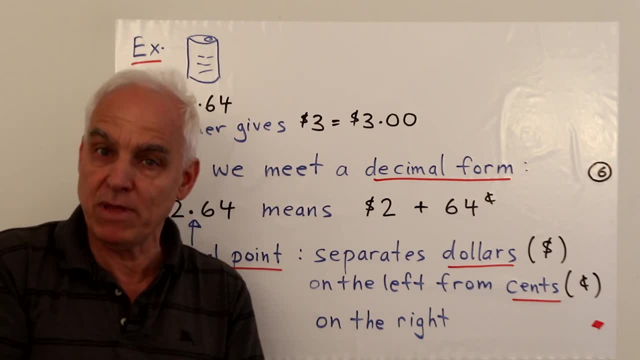 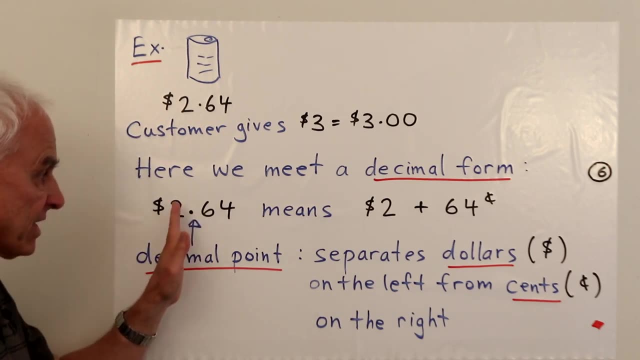 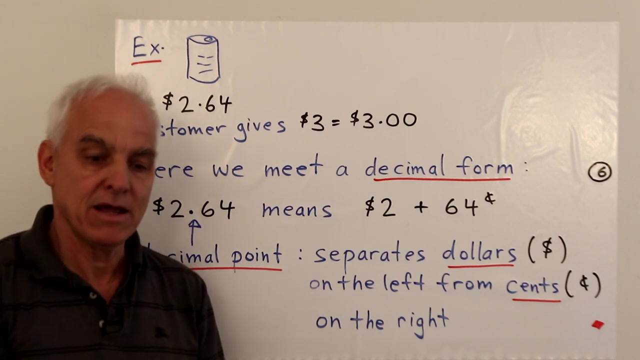 mathematical representation of money that students have to become familiar with. this decimal point here in the context of money separates dollars on the left with cents on the right, and typically there's always two places on the on the right because it's always a number of cents between zero and 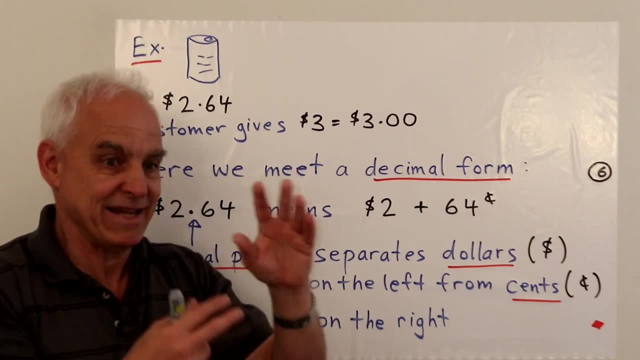 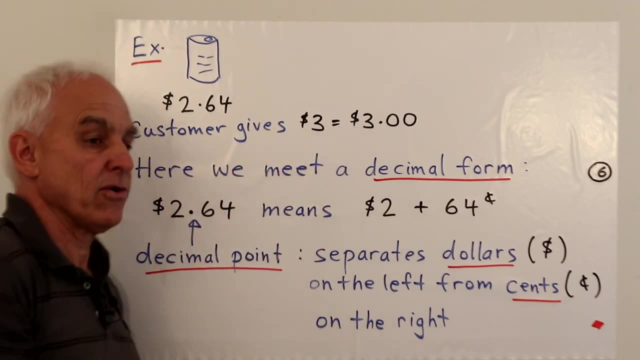 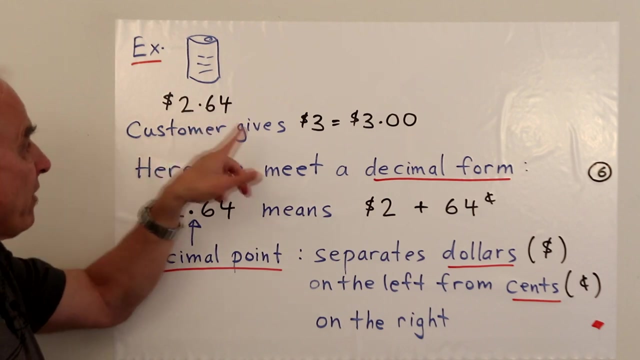 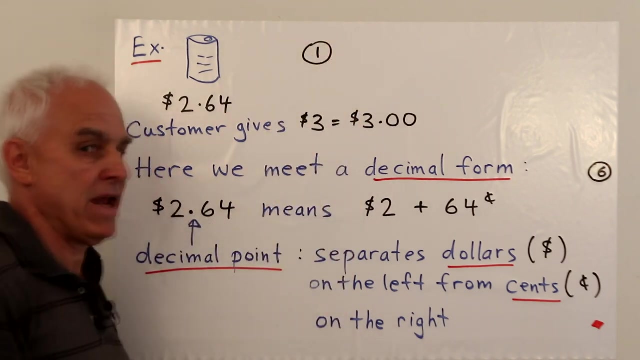 99. so there's two decimal places. we say okay. so let's work out what happens. if, say, the customer gives three dollars for this drink. we have to get some change. how do we add up, count up from two dollars and sixty four to three dollars? well, we're gonna add a penny or one cent, assuming. 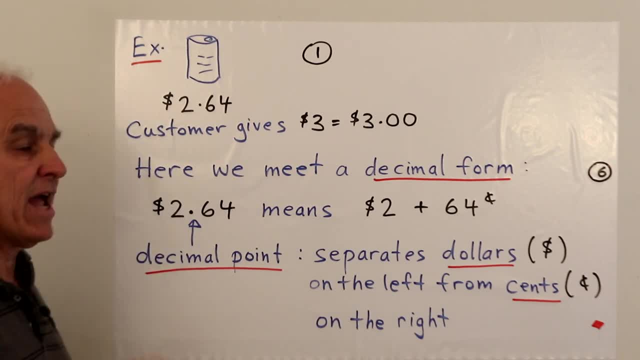 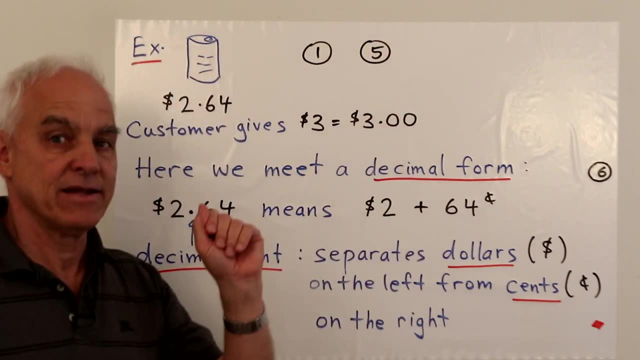 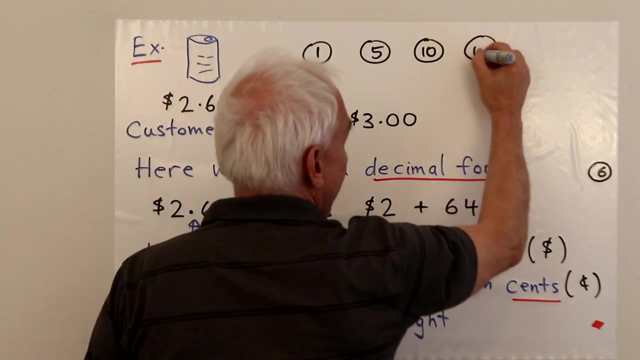 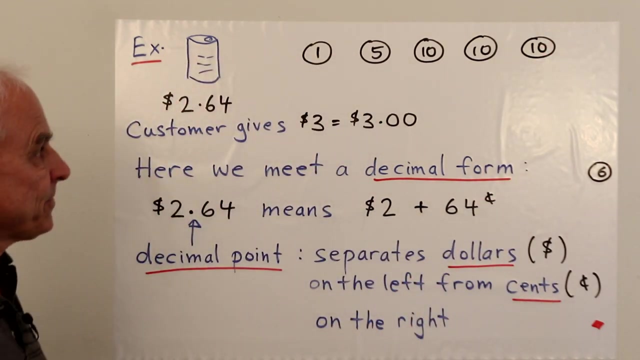 we have such a thing available. so that makes two dollars and sixty five. then we add five cents, that's two dollars and seventy, and then ten cents makes two dollars and eighty. another ten cents makes two dollars and ninety. another ten cents makes three dollars. so the total amount of change is one plus five plus. 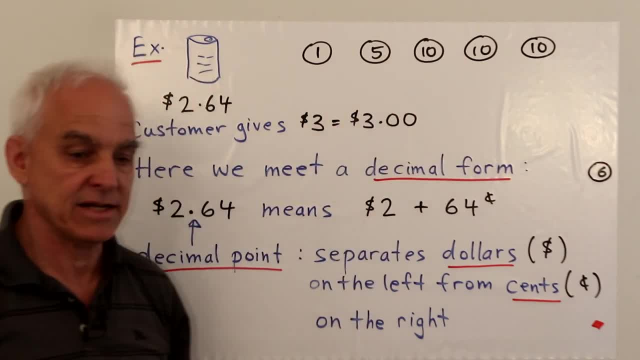 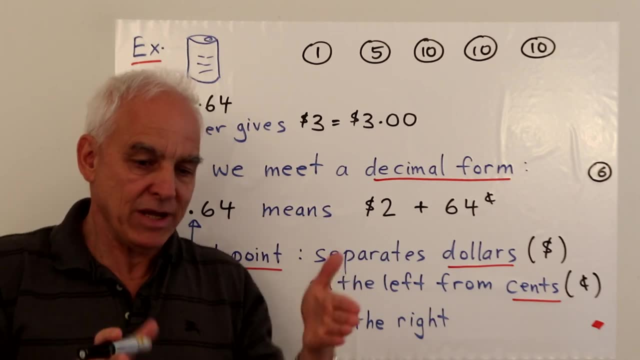 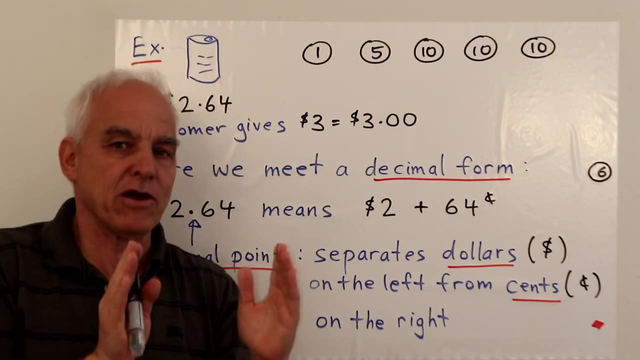 ten plus ten plus ten, which is thirty six cents change. okay, so this is actually quite important because it's an opportunity for us to introduce in a very concrete way the idea of a decimal number, admittedly in a very special context. okay, we don't have to say 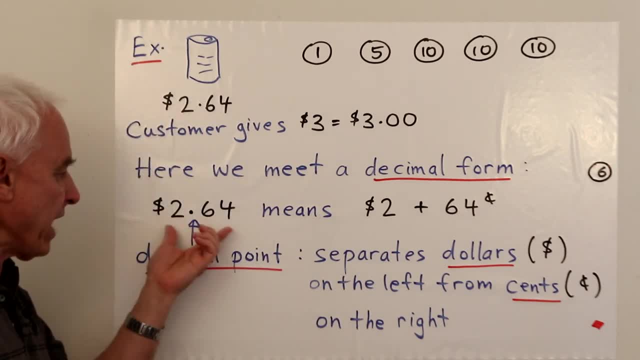 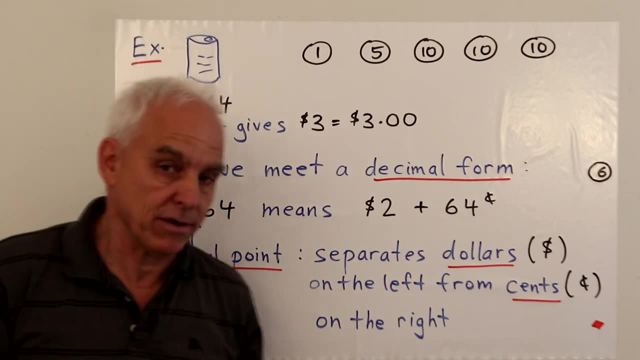 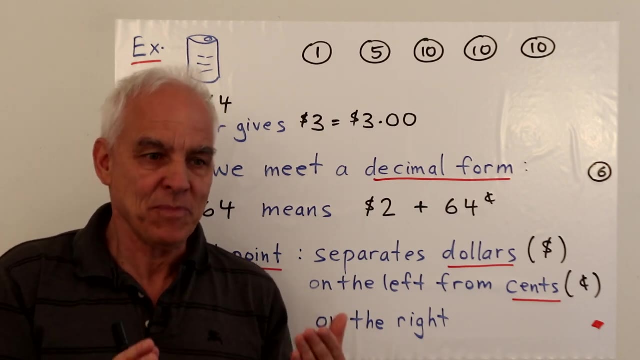 much about it. we're just introducing this way of representing a certain amount of money that has both dollars and cents involved, and this will be very familiar to young people because everybody has gone to stores and seen the price of things. so this is a a comfortable, familiar kind of number. 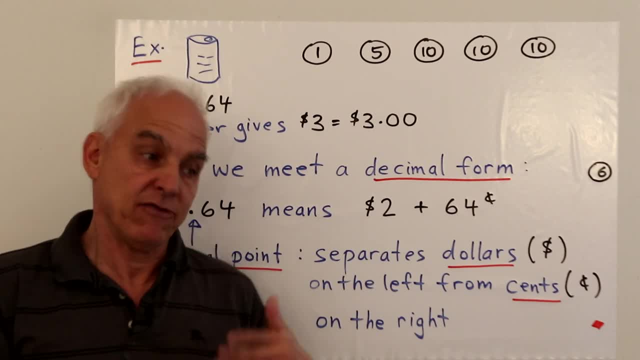 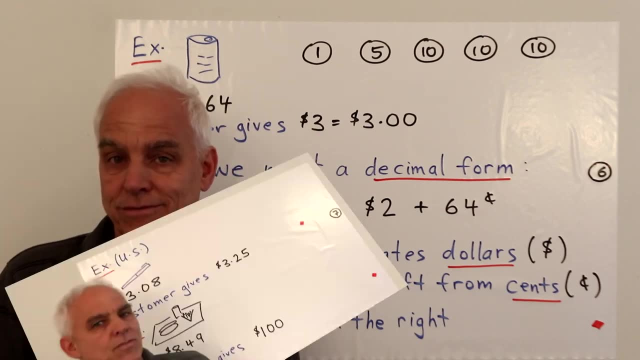 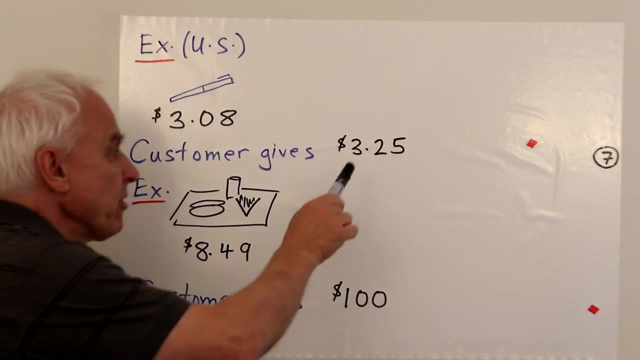 that they know the meaning of it, they know what this means, okay, and they have to be able to work with it, understand what's, what's going on, how to make this kind of computation, for example, is useful. here's another example: a pen costs three dollars and eight cents, and, let's say, a customer. 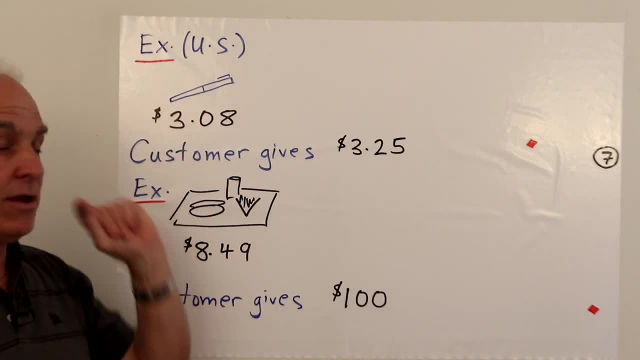 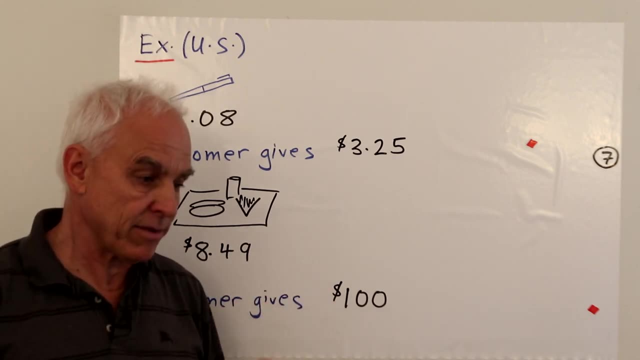 pays three dollars and 25 cents. so this might happen in the united states, where there's quarters representing 25 cents. wouldn't happen in australia. in australia you'd pay with three dollars and 20 or maybe three dollars and fifty cents. so suppose we paid with three dollars and 25 cents, so we have. 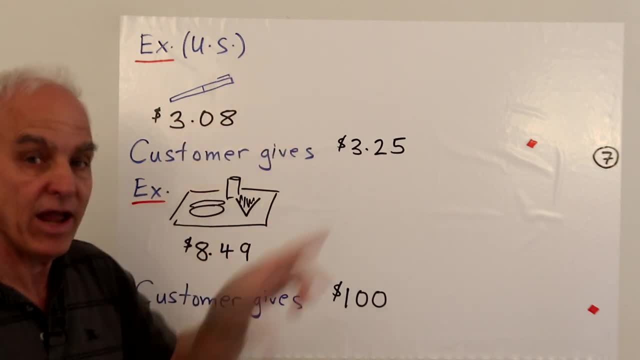 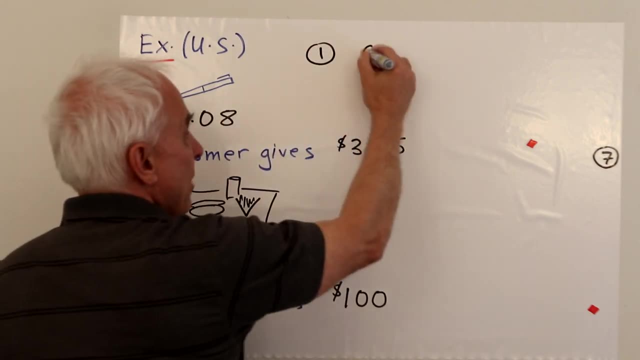 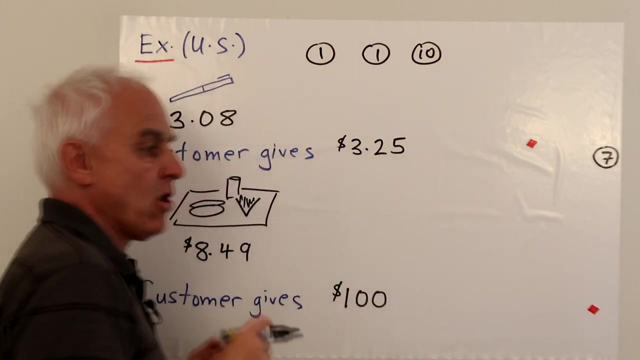 to count up from three dollars and eight cents to three dollars and 25 cents. of course that's not too hard to do. three dollars and eight plus one is three dollars, and nine plus one is three dollars and ten, and then the next natural unit might be ten. so that's three dollars and twenty. and now 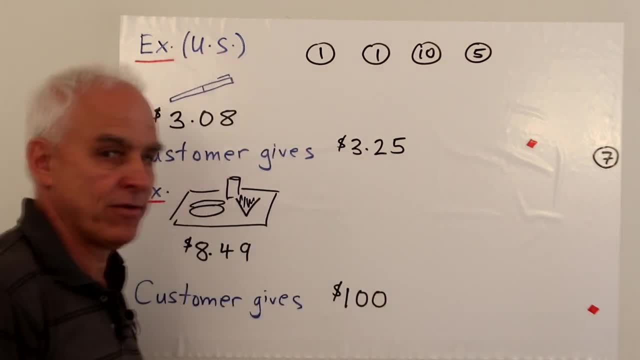 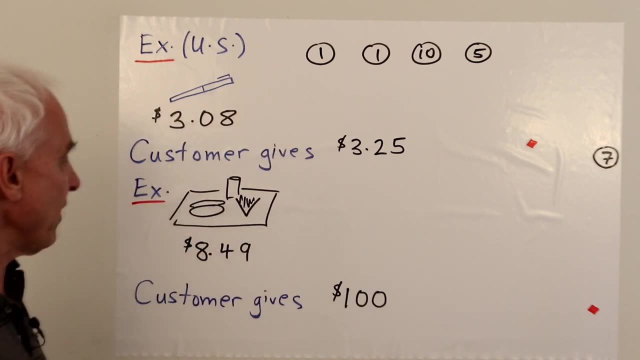 we add another five, that's three dollars and twenty five. that's the amount of money we're going to need. change received: We buy the pen for $3.08 with $3.25.. Here's another example. Here's some kind of fast food meal which costs $8.49.. And the customer only has a $100 bill. So we have to. 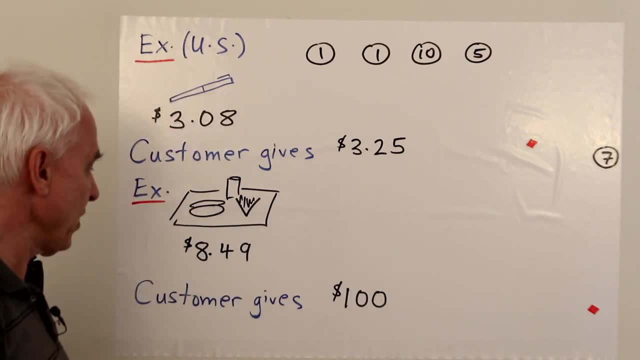 give them change. but we have to be careful because this is quite a lot of money involved. Okay, so let's do it. Let's count up from $8.49 to $100.. Okay so we work on the cents first. 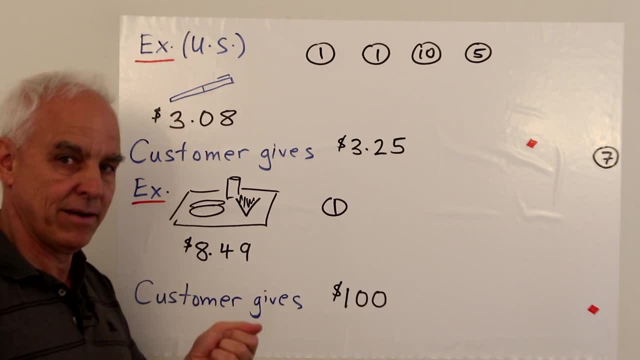 One cent added to this makes $8.50.. Okay, $8.50.. Now we're going to add 50 cents to that. $8.50 plus 50 is $9.. Okay, and now we switch to dollars. $9 plus $1 is. 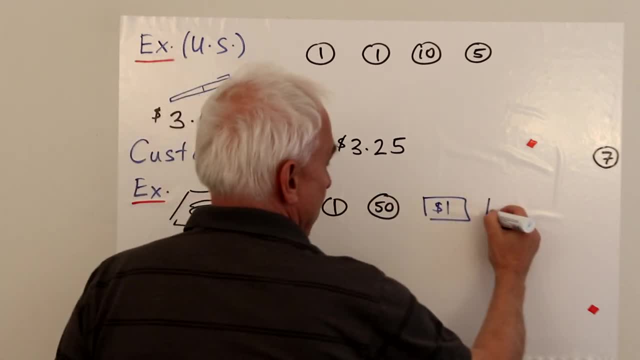 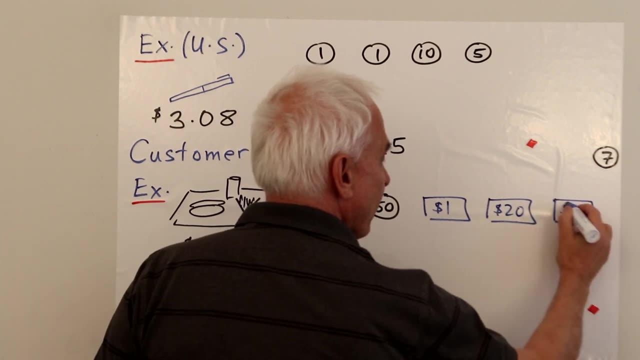 $9.50.. Okay, so we work on the cents. first, One cent added to this makes $8.50.. Okay, and now we $10. And maybe we'll suppose we have $20.. That makes $30.. Another $20 makes. 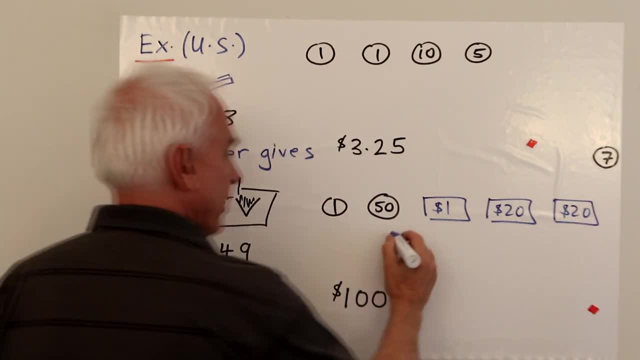 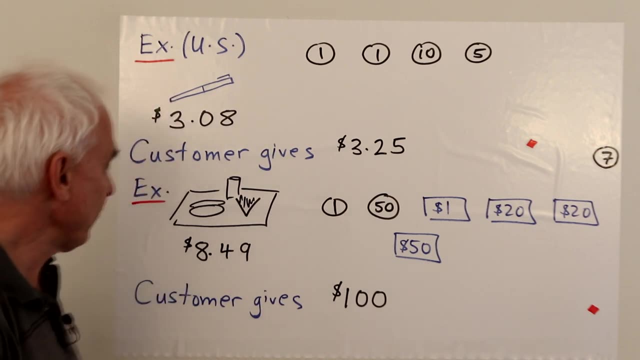 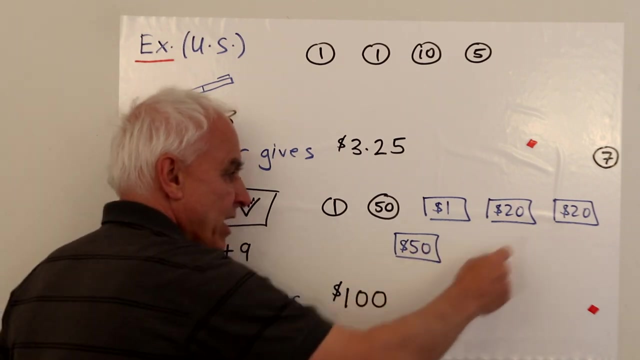 $50.. And then one more $50 bill will total us to $100. So let's review that $8.49 plus one cent is $8.50 plus 50 cents is $9 plus one is $10 plus 20 is $30 plus 20 is $50 plus 50 is $100. 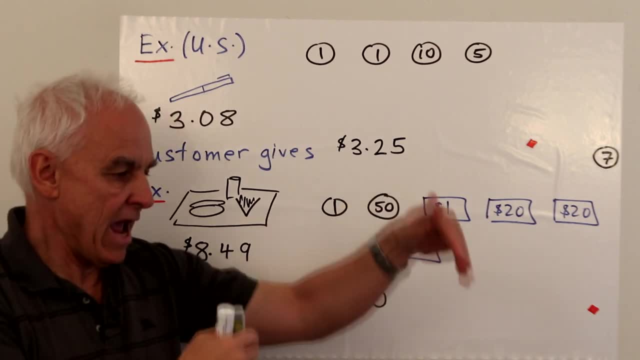 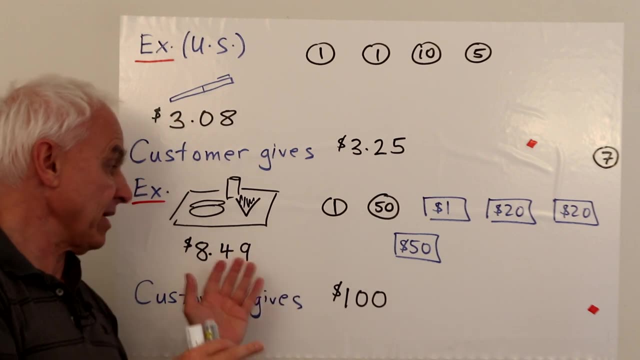 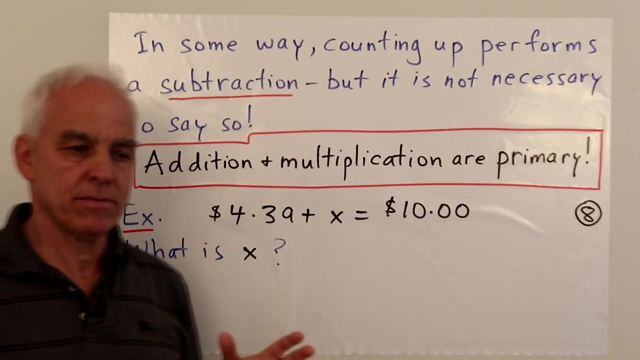 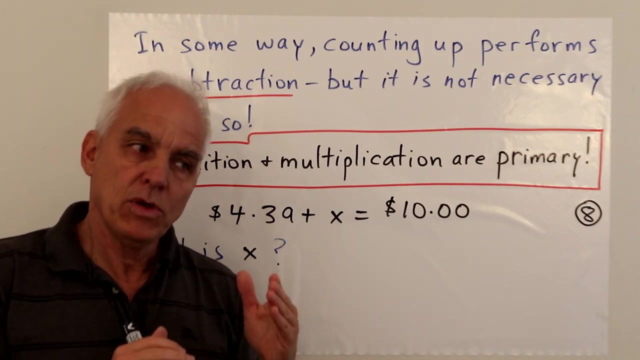 So we're utilizing this ability to be able to add sequentially, but actually also traversing the divide or the separation between the cents on the right-hand side and the dollars on the left-hand side. So in some way counting up performs a subtraction, But it's not necessary to say it in those words, So we do not need to know. 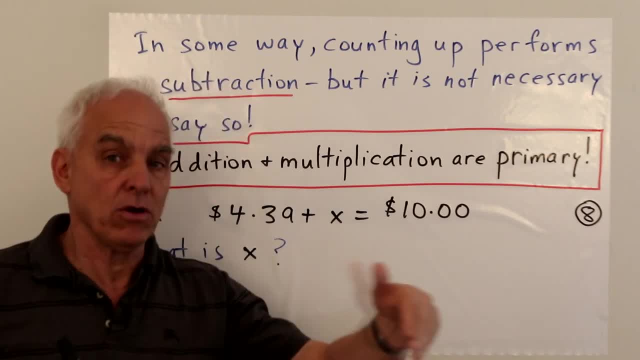 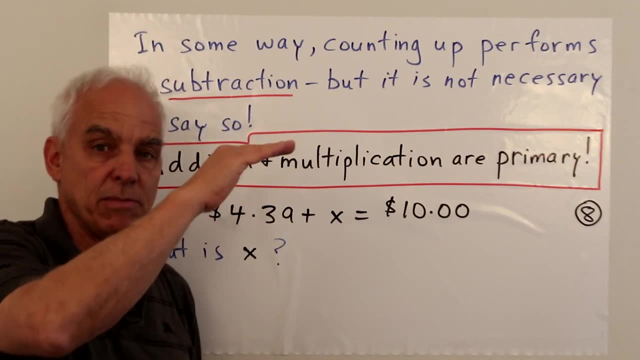 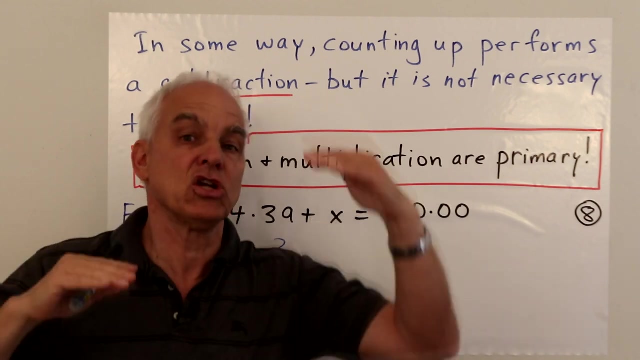 what the operation of subtraction is, to be able to follow this discussion, And I think it's important to elevate addition, to be at a much more primary and important level than subtraction. So for me those two things are not equal. Okay, addition is much more important than subtraction. 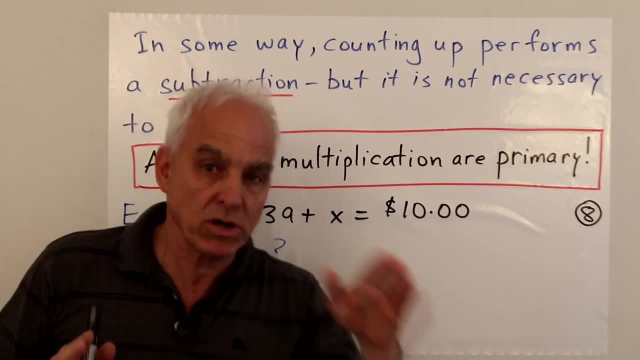 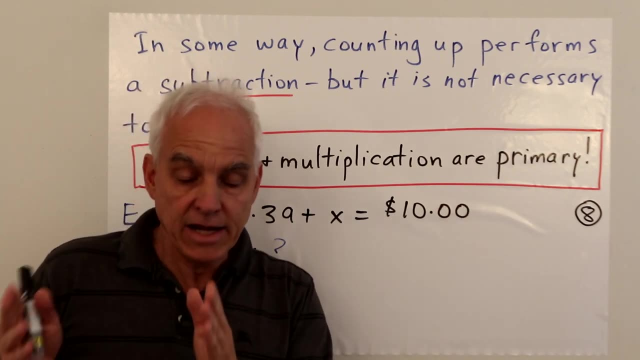 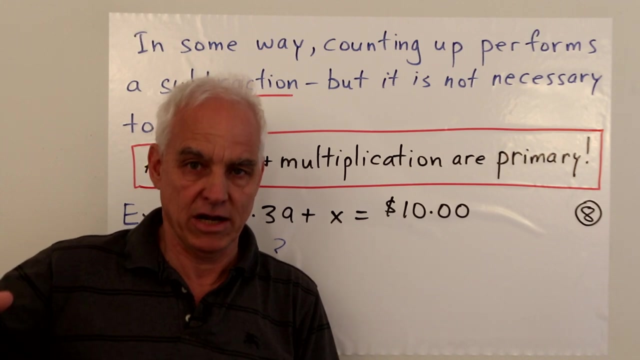 Ar mathematically, And young people should spend more time on addition. If they get addition down really well, then subtraction is a lot easier And it's in any case a secondary operation that has all kinds of additional difficulties associated with it. In the same way, multiplication is primary. 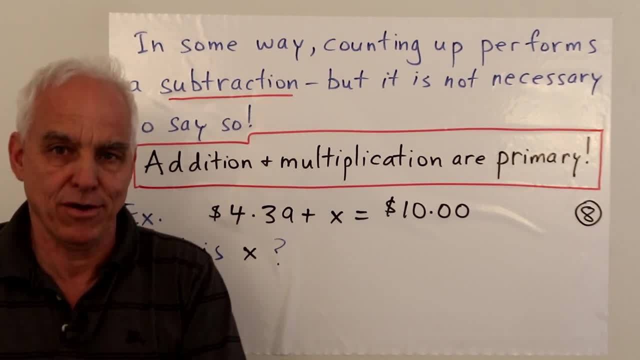 while division is a kind of a secondary, more complicated thing. Okay. so addition and multiplication, in my view, are the two things that make a thing. Okay. So addition and multiplication, in my view, are the two things that make a thing. Okay. So addition and multiplication, in my view, are the two things that make a 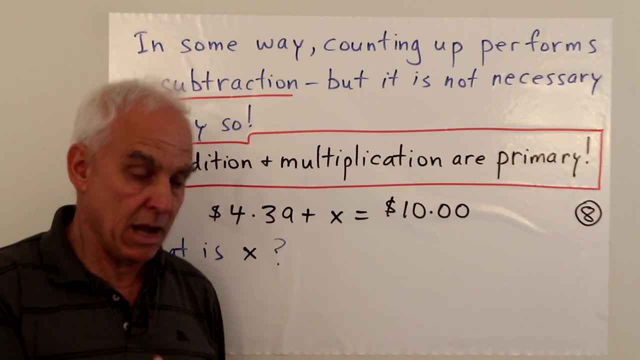 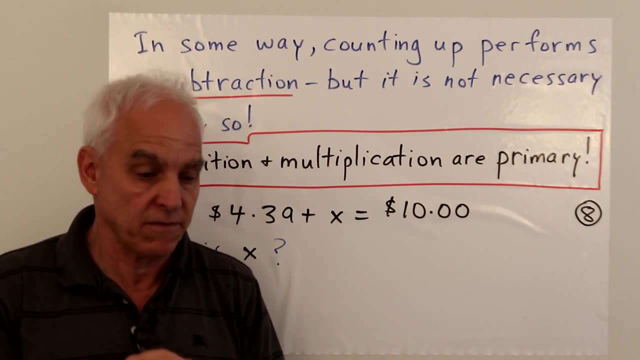 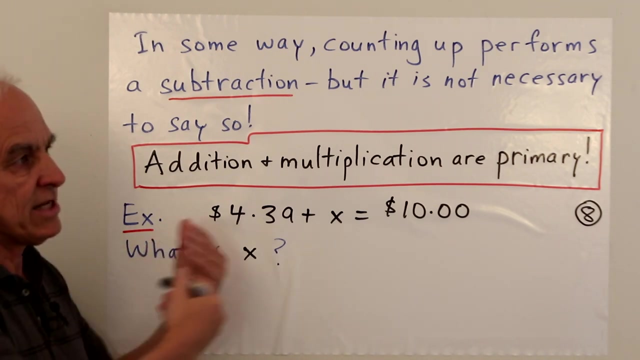 two main operations that especially young people should become familiar. that's sort of. the first order of business is to establish those two operations on a very solid footing. okay so, but in in fact we are also doing kind of subtraction and we can use this technique of counting up to solve problems which otherwise you might think we need subtraction for. 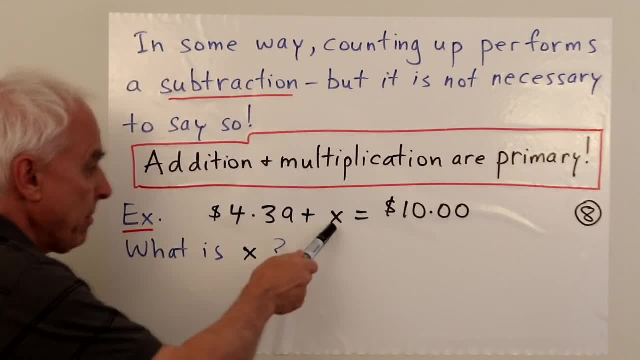 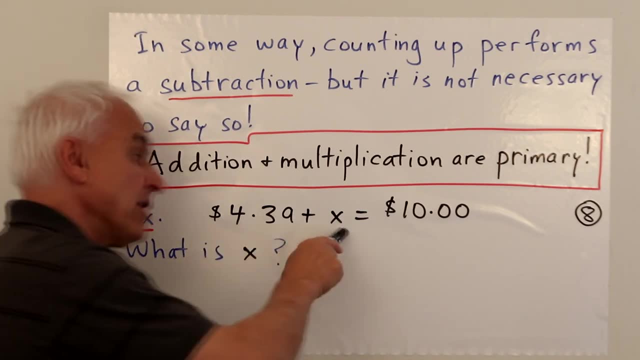 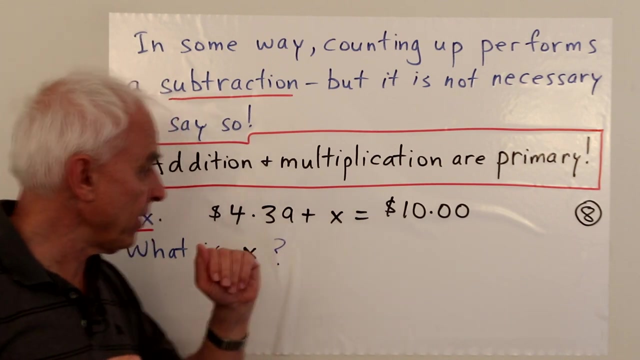 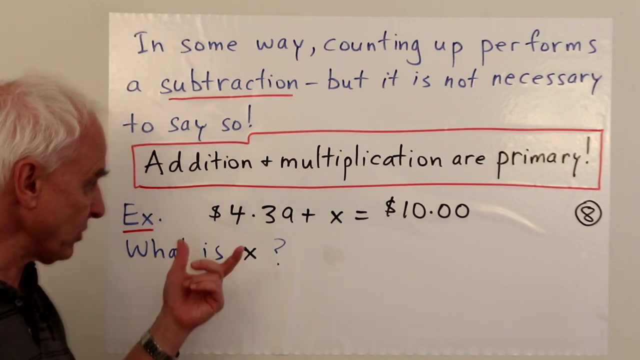 for example, there is some mystery amount of money, x, which has the property that four dollars and thirty nine cents added to x makes ten dollars. what is x? can we solve this equation for the unknown x? so we can try to solve this by counting up from four dollars and thirty nine to ten dollars. 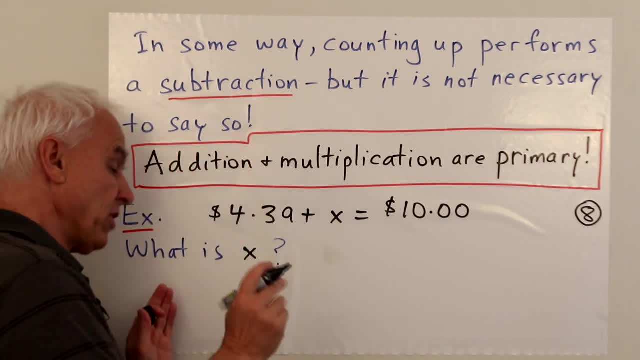 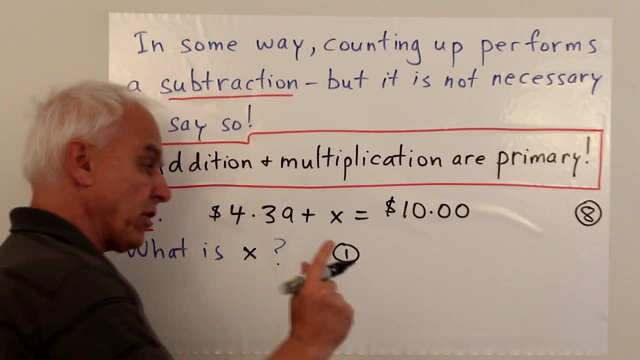 so let's do that in the same way that i did before. so we'll start with four dollars and 39 and ask: how much do we have to add to that? so first of all let's add one that makes four dollars and 40, then we'll add 10 that makes four. 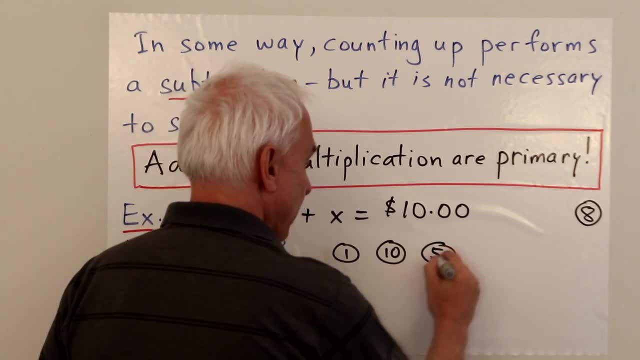 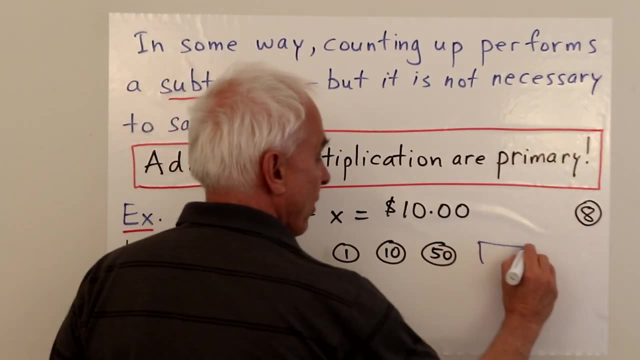 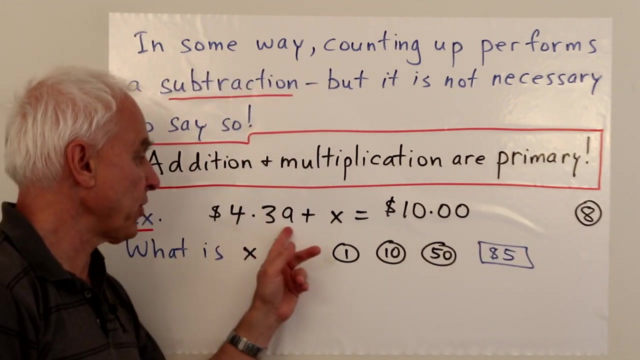 dollars and fifty, and then we'll add 50, and that makes five dollars, and then we have to add another five dollars to get up to ten dollars. so i'll write it like this: okay, so this is what we've added to: four dollars and thirty nine. 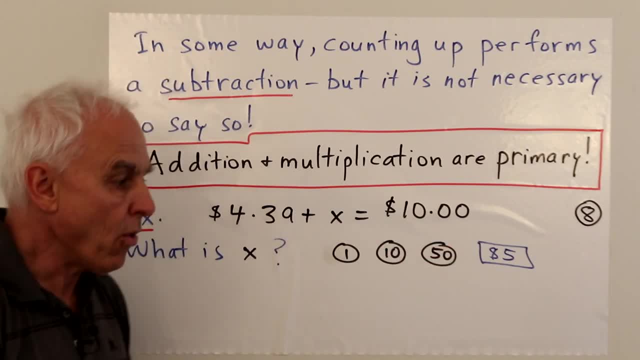 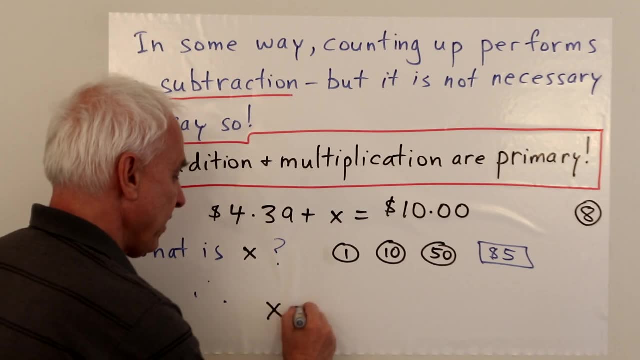 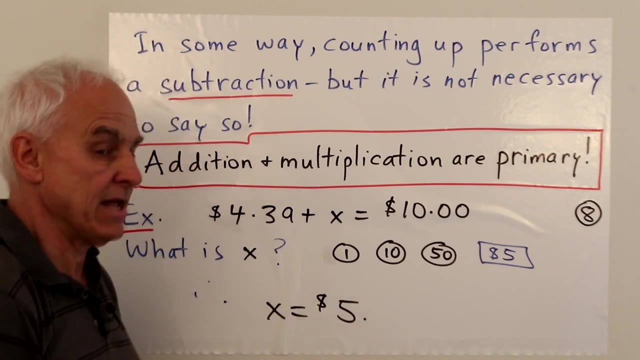 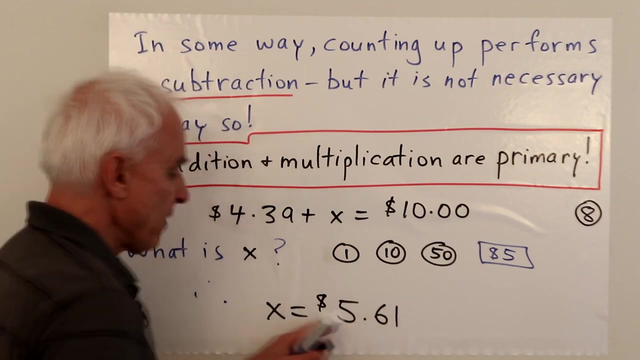 to get ten dollars. so we can conclude that the x is really this total that we have here all together. we've added the five dollars. comes first five dollars, and how many cents? one plus ten is eleven plus fifty is sixty one. so sixty one cents five dollars and sixty one cents. 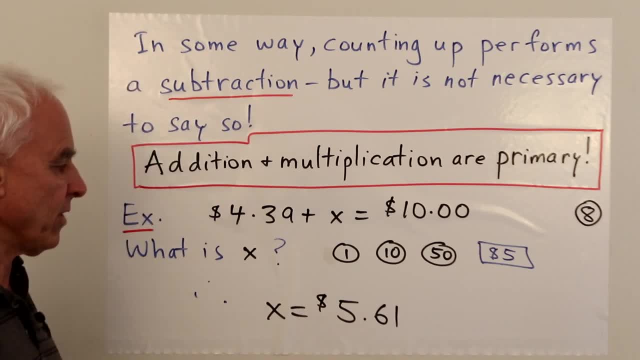 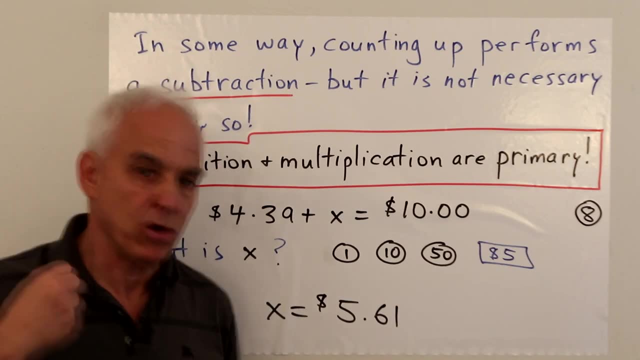 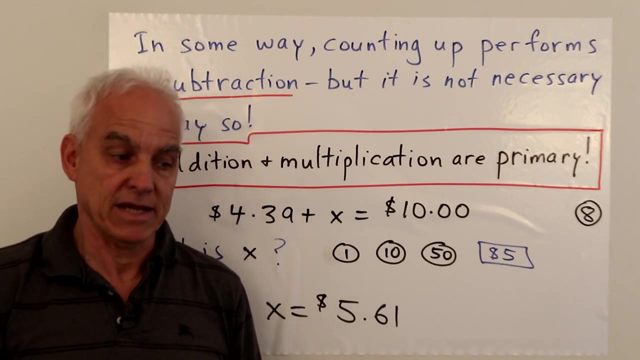 is what x has to be. so we've done a kind of subtraction problem, but without subtracting we've been able to employ this counting up procedure to actually get an answer to this problem. so it means that young people can do this with just their additive skills. and finally, i just 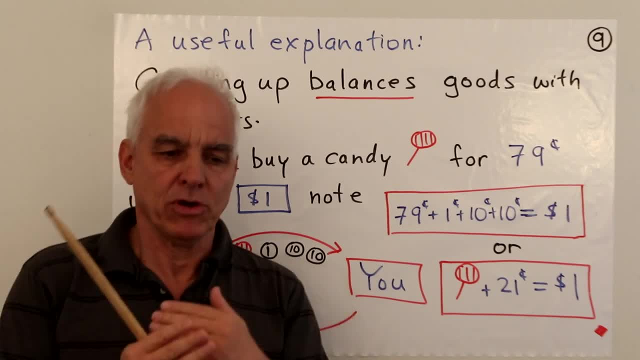 want to point out that one way of thinking about what we're doing here, with this counting up, is that we're balancing things. okay, that's a nice way of thinking about it and apparently i told you actually the next chapter- it did make that that without不會. 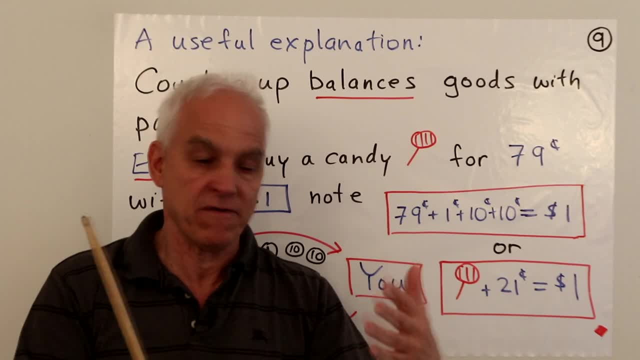 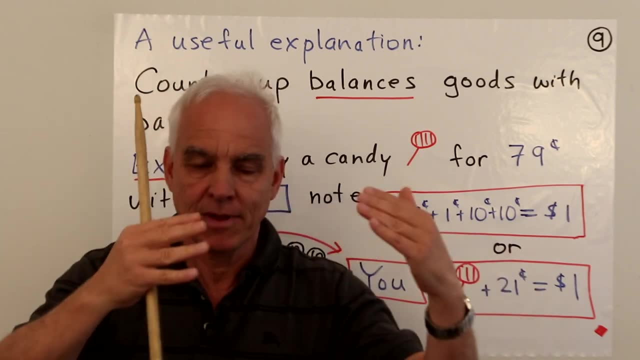 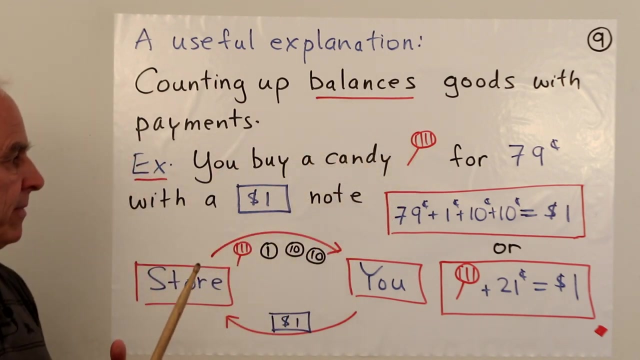 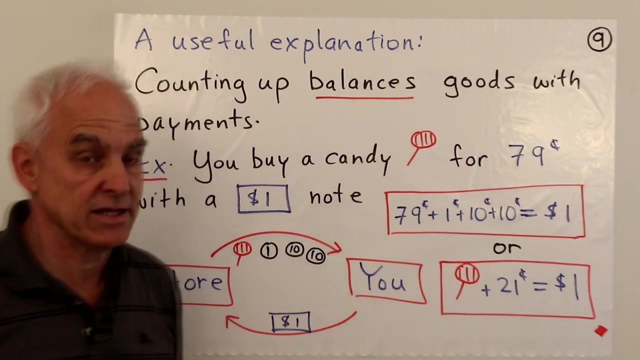 because balancing connects with equations which are fundamental objects, fundamental kind of way of thinking in mathematics. so the idea of balancing and what's happening here is that the counting up balances the goods with the payments. let me illustrate that by going back to our first example. we bought a candy which is costing 79 cents and we've paid with a one dollar. 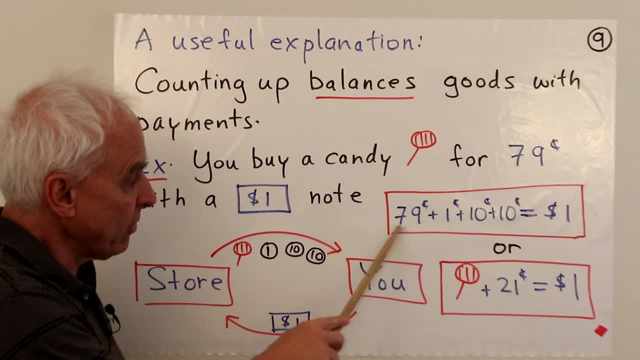 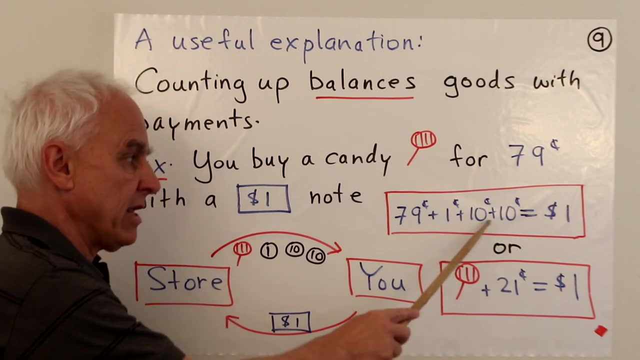 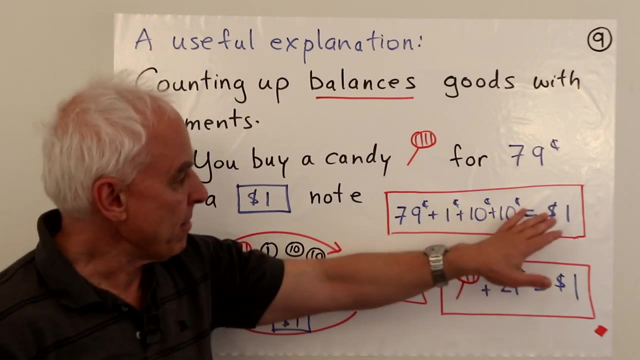 note and we've counted up and determined that, with 79 cents to start with, we should get one cent back for a total of 80, plus another 10 cents, for a total of 90, plus another 10 cents, for a total of a hundred cents, which is the same as one dollar. all right, so this is the mathematical kind. 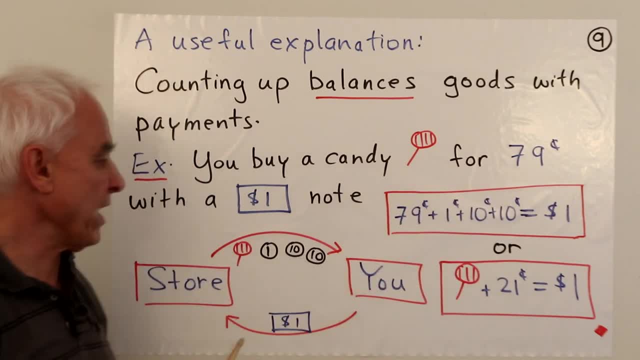 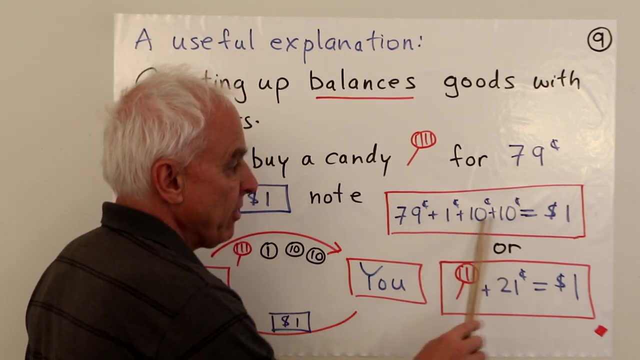 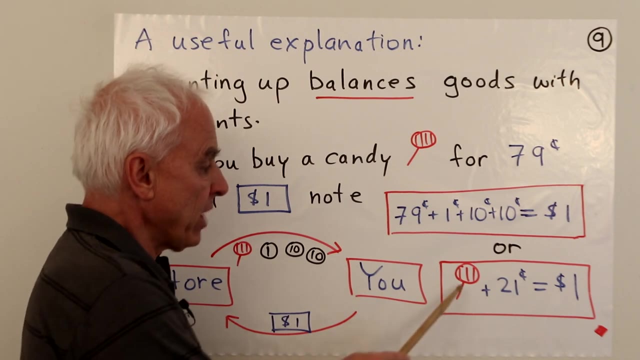 of equation that represents what's actually happened, and we could lump all this together. so the one plus ten plus ten, that's actual amount of change that we've received back. that's a total of 21.. so we could rewrite this and say that, okay, the candy plus 21 cents amounts to the one dollar, and i want you to think about that. 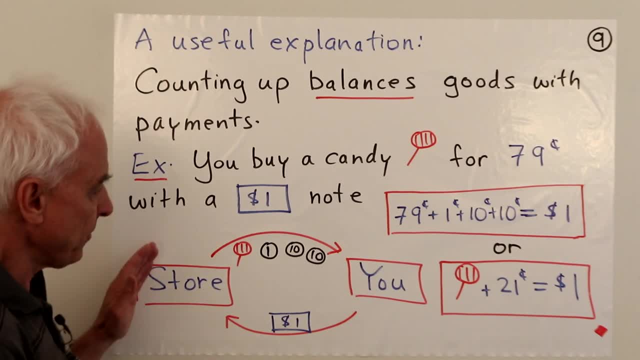 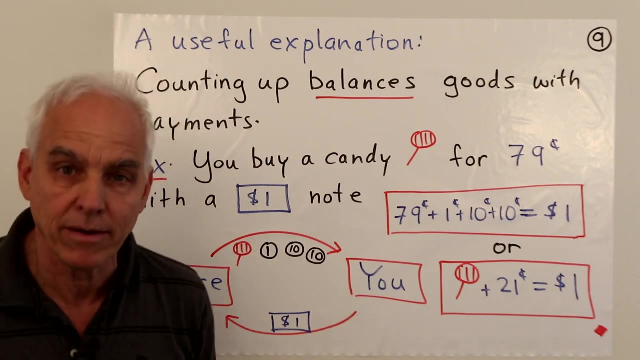 in terms of the sort of balance that there's things that are going from the store to you- you're the one buying the candy, let's suppose- and there's something going from you to the store, so you have paid the store one dollar, so one dollar has gone from you to the store. on the other hand, 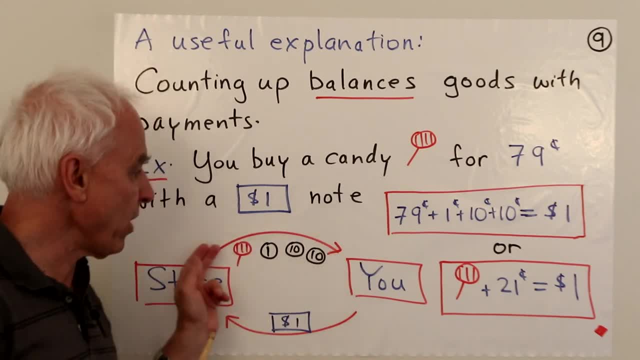 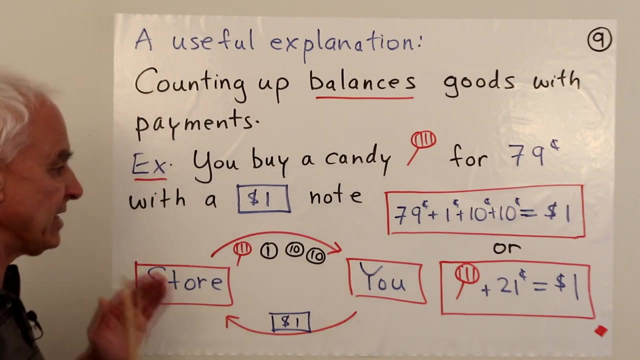 the store has given something back. the store has given you, first of all, the candy, that's the main thing, but then also this additional change, the one, the ten, the ten cent coins. okay, so you've received this, you've given this, and the idea is that these things balance. okay, the total amount that the 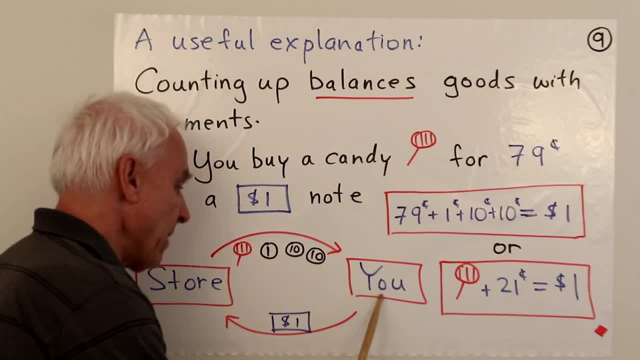 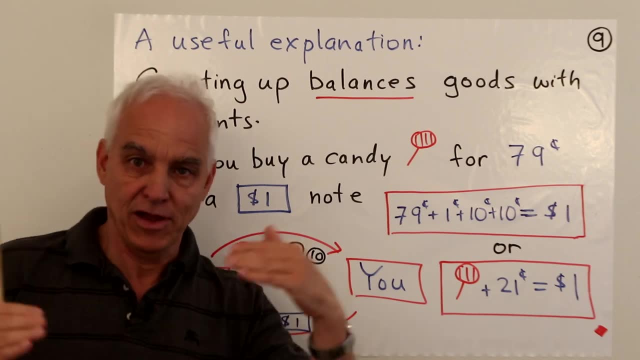 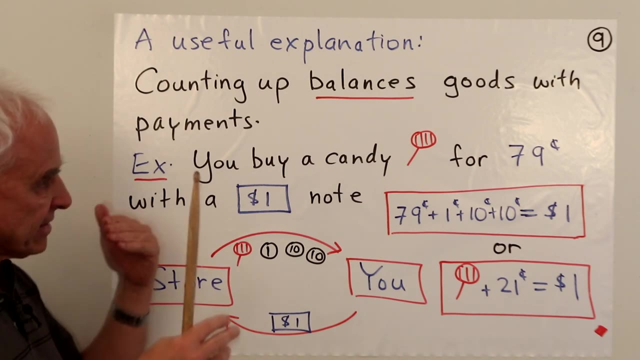 store has given you equals the total amount that you have given to the store. things are balanced. there's a sense of fairness and rightness in this transaction. so this kind of thing i think students can can see, so they get the sense that, yes, that things are fair, the amount going in this direction,